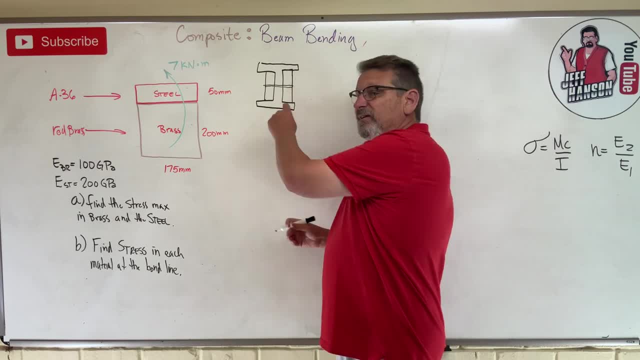 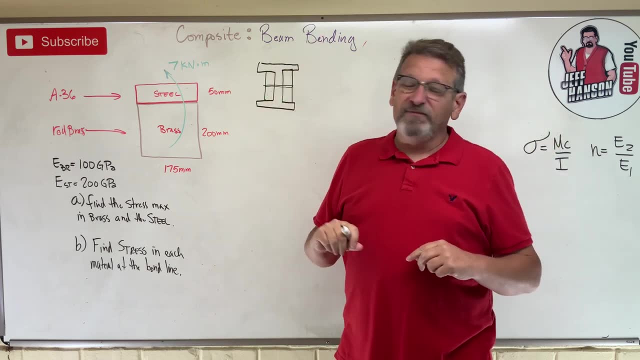 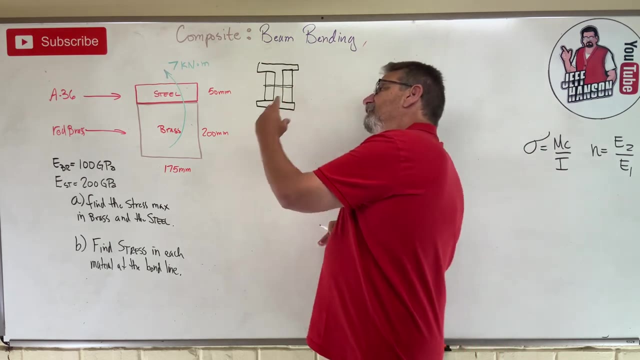 have and make a composite beam. Now I've got the steel strong to carry the load and then I've got this wood that I can nail to right. So this is a common thing used in construction, for houses and such. okay, When do we use steel bonded to brass? I don't know. okay, Don't get me on that. We're. 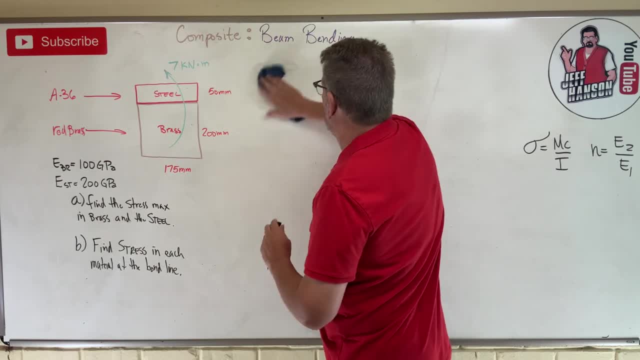 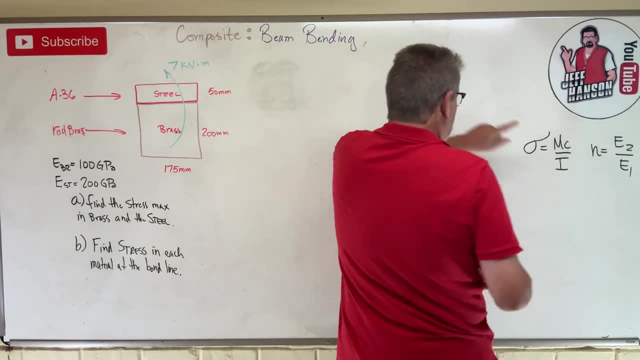 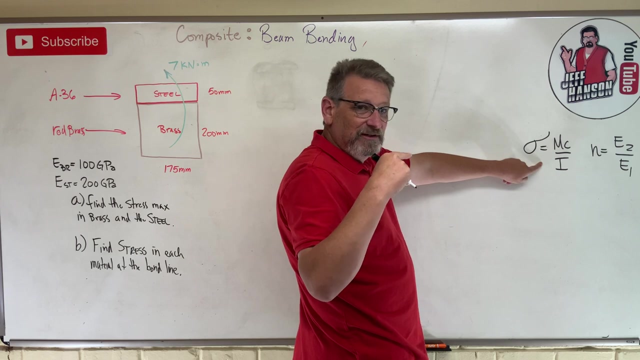 just making this up. We'll see if we can figure out how to do it. If you ever had to do it now, you will know how. Okay. so here's the deal. If this equation is only built to handle one material at a time, then let's trick this equation and let's make that beam into one material. okay, I'm. 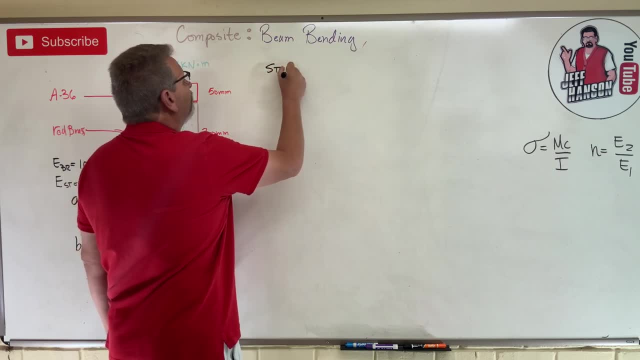 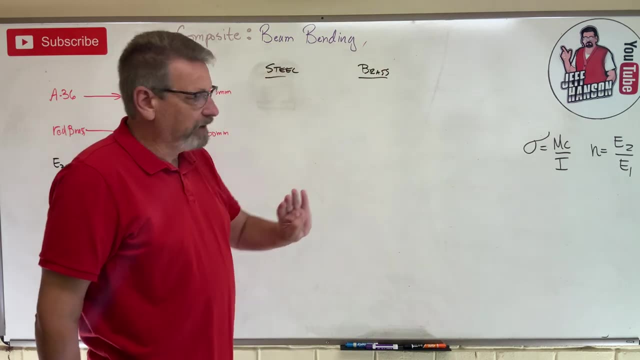 going to put two things up here. I'm going to put steel and I'm going to put brass. okay, Now, here's what I'm going to tell you. okay, What we have to do is we have to do one of two things. 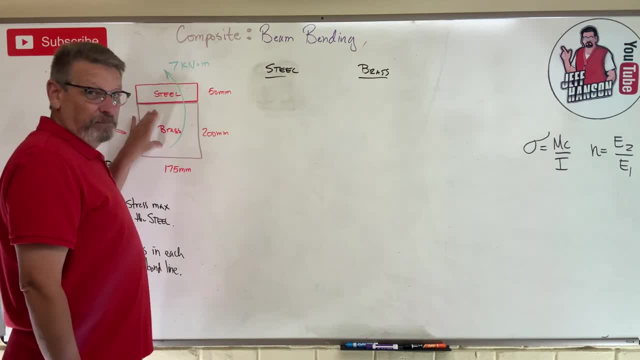 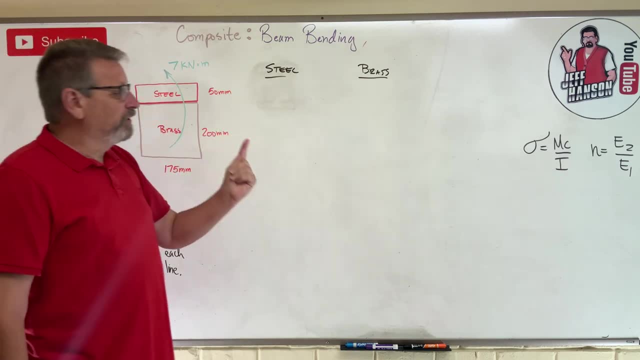 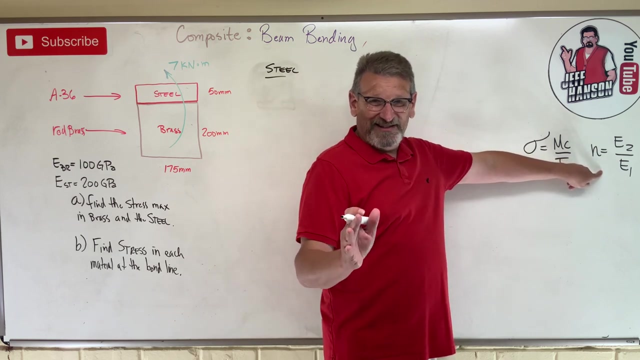 We have to either convert this whole beam into brass or convert the whole beam into steel, And to convert one material into the other. we have this little easy equation over here, And all it is is a ratio of the modulus of elasticities. okay, That's all it is. 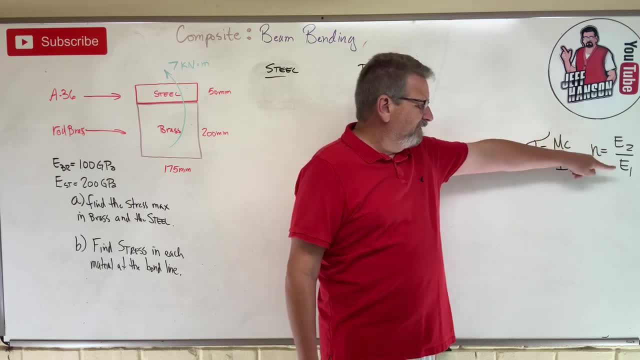 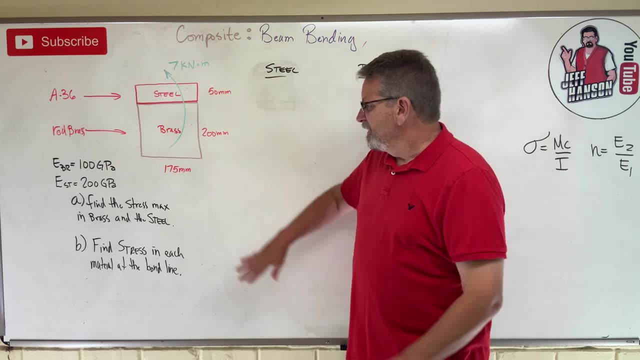 So n equals material. one divided by material, two or two divided by one, whatever, okay, And you're just, and you're like which one goes where? okay, So here we have steel and brass and we have the modulus of elasticity for steel and brass. Well, here's how I like to do it, okay. 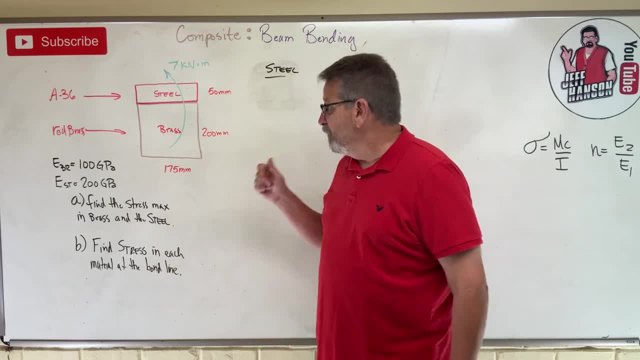 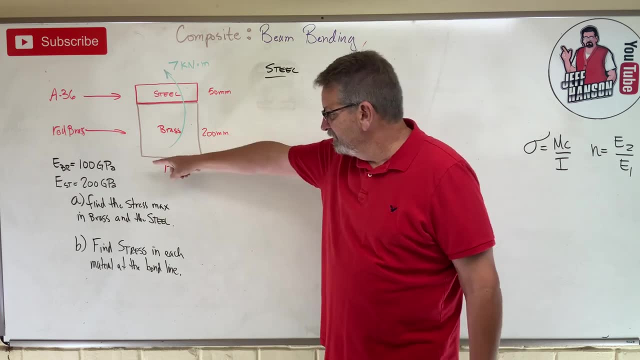 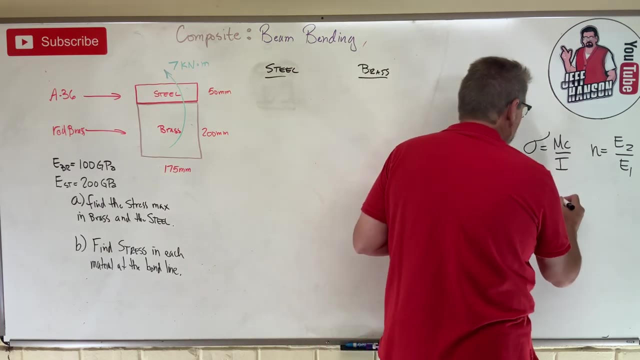 I always like to put the strongest material on the top. Now we know- I hope we know- between steel and brass who's the strongest Steel, right Matter of fact, it's about two times as strong, isn't it? So that's exactly what we're going to get over here. We're going to get n is equal to. 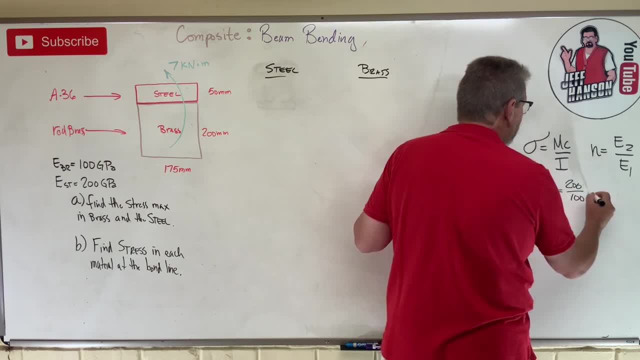 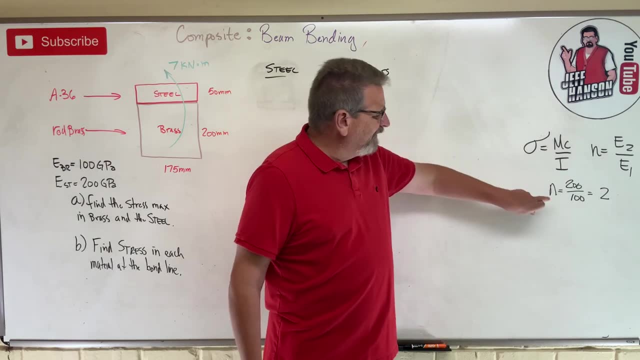 200 divided by 100, which is equal to two. I always like to put the strongest material on the top, and that way n is going to be the strongest material on the top. So I'm going to put the strongest material on the top. So I'm going to put the strongest material on the top, and that way. 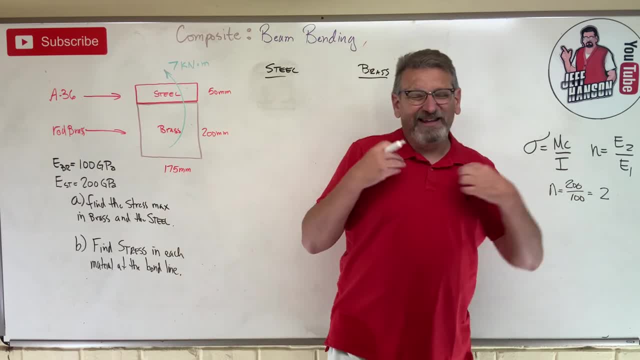 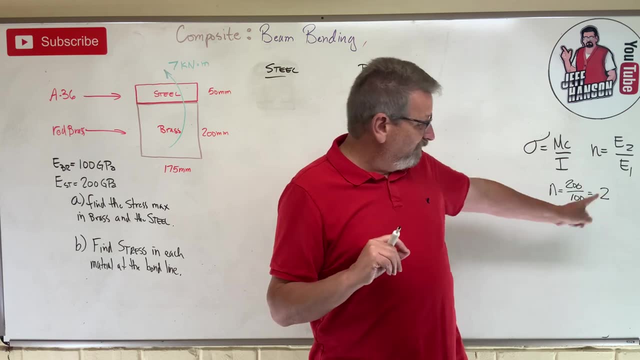 n always comes out to a number bigger than one, And what I tell myself is: oh, that number that I get for n, whether it's 1.3 or 2.7, or, in this case, just two, that means that this material is. 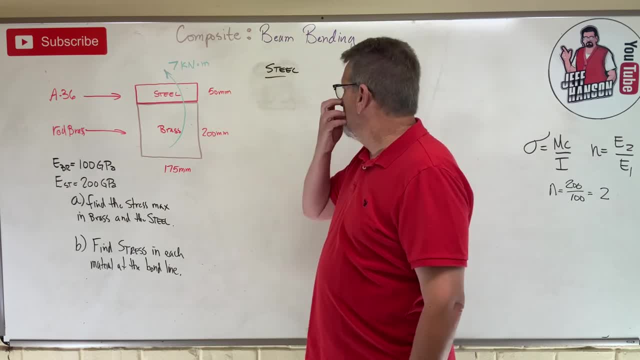 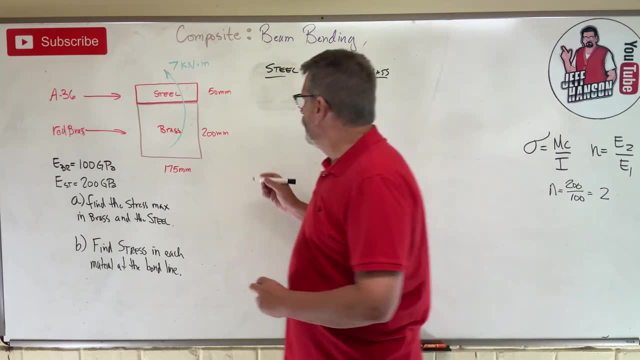 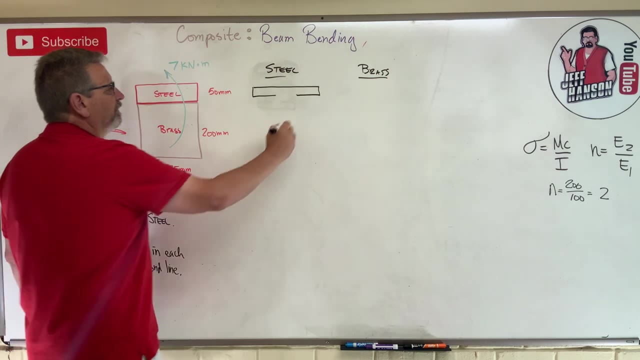 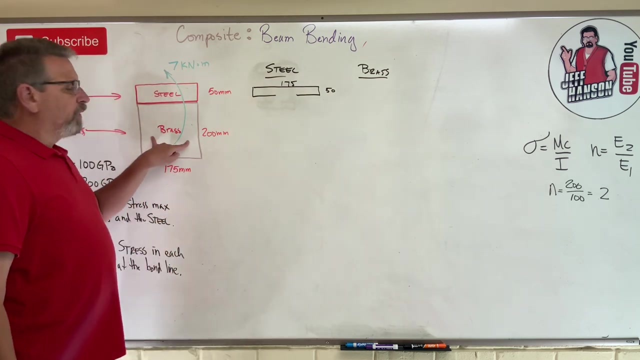 two times as strong as that material. okay. So if we turn this whole beam into a steel beam, what would it look like? okay, Well, number one: the steel is unchanged. There, it is okay. It's still 50 by what? 175, okay, But what do we do if we replace this brass with steel? 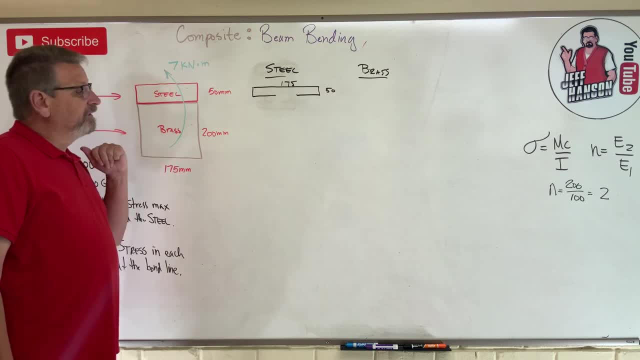 what happens? Do I need this much? No, As a matter of fact, I only need half as much to be as strong as the steel, because the steel is twice as strong, And so what I wind up with is something like this: 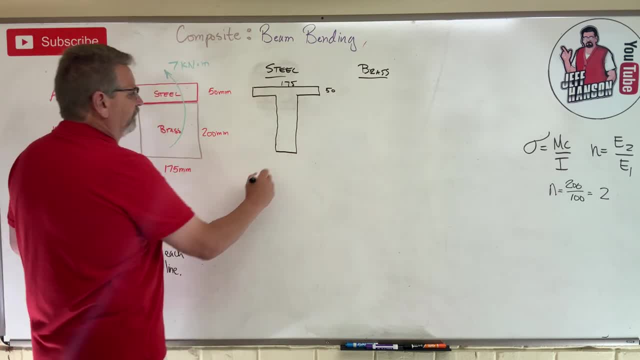 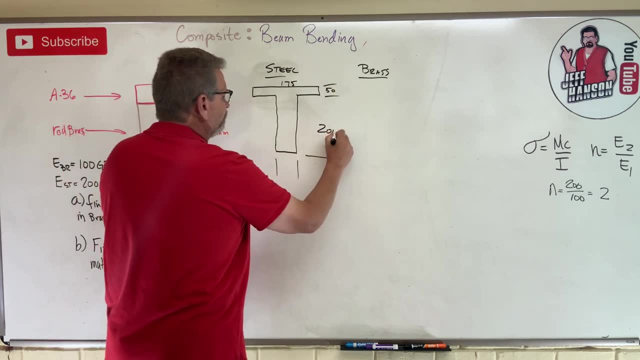 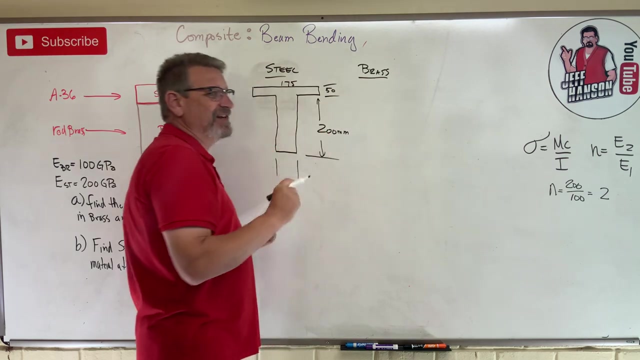 okay, What is this? Let's see this right here. well, this right here. okay, Now here's the important part. This is still 200, okay, You cannot change the height of the beam. You can't change the height. 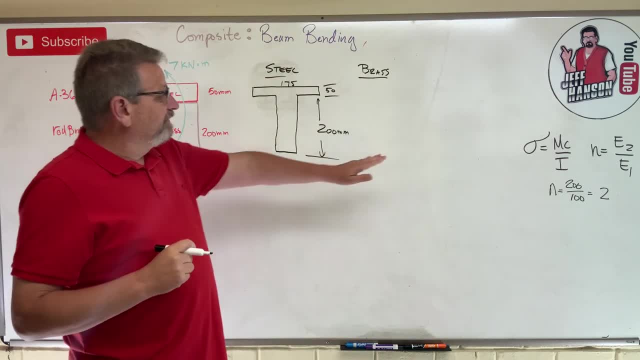 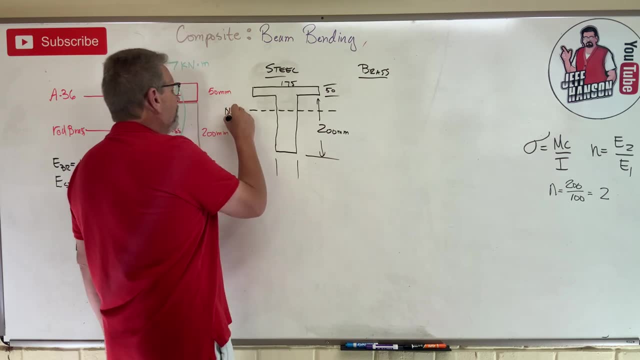 okay, You can't do it, But notice, and this is quick because look here's, when I have the neutral axis, let's say the neutral axis is right there. okay, In A, okay, I have C, which is the. 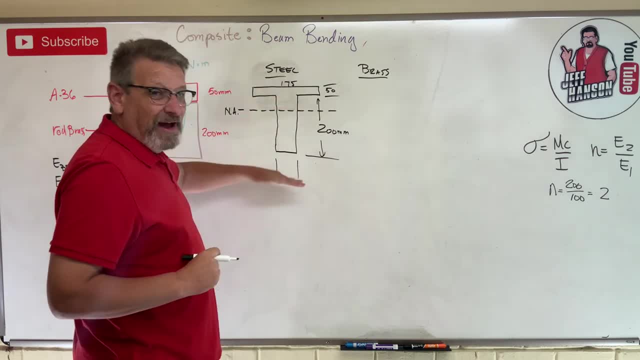 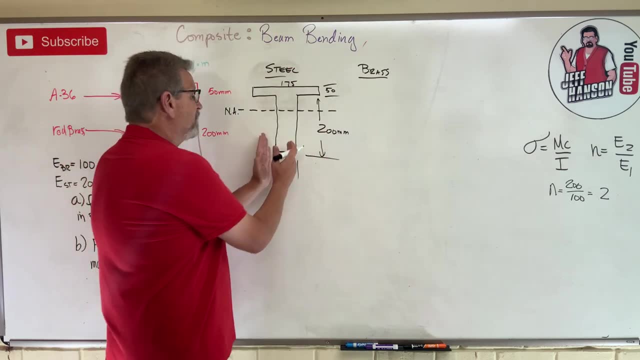 distance from the neutral axis. I have C, which is the distance from the neutral axis. I have C to the outside of the part, right. So C depends on up and down distance. It doesn't depend on left and right distance. So I get this transformed part can be as wide or skinny as I need it to be. 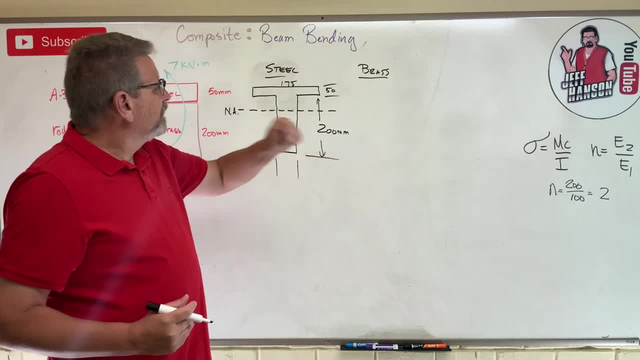 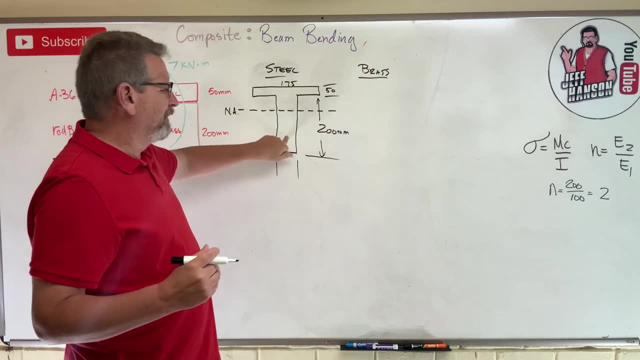 and it won't affect that equation over there. okay. So here's the deal. I decided that I only need half as much brass, since steel is twice as strong as brass, And so what's this width right here? Well, it's 175.. 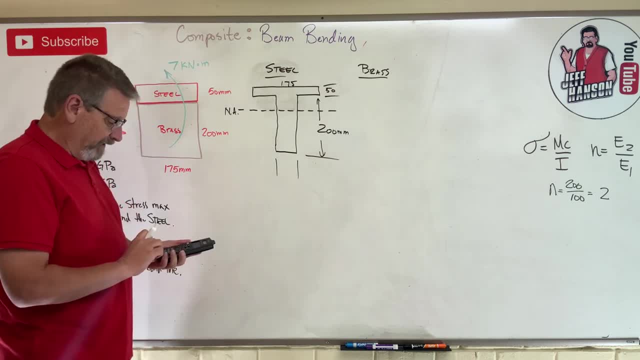 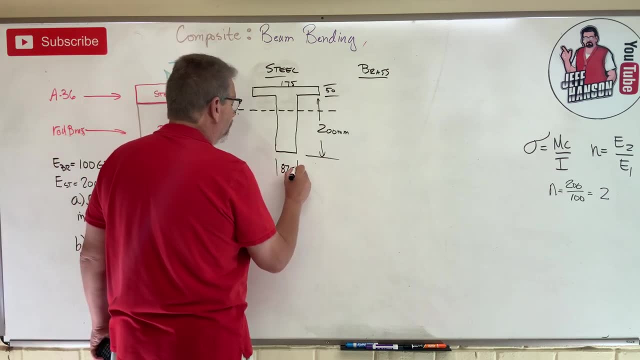 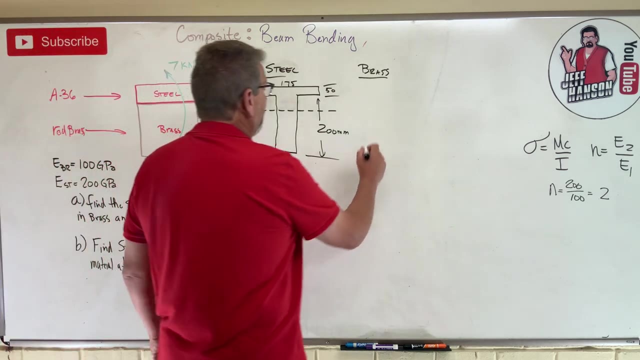 175 divided by 2.. What is that? 87.5, 175 divided by 2,? 87.5, okay, But what if we wanted to convert the steel into brass? okay? Well then I would have this: There's the brass, okay. Now. 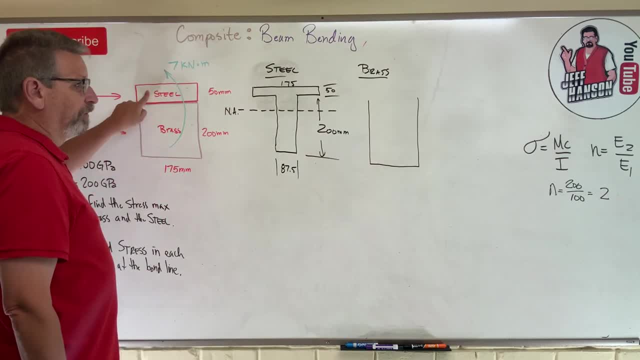 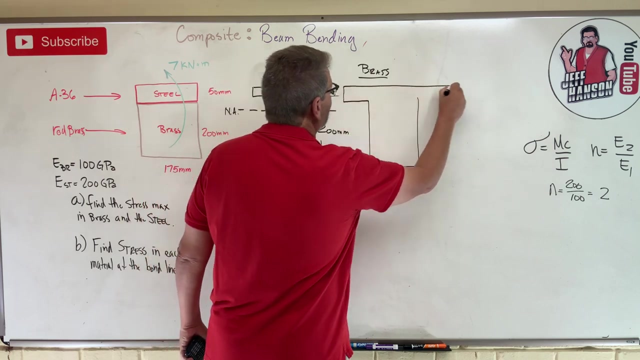 to do that much steel. what do I need? If I'm going to replace that steel with brass, I need twice as much of it, right? Because the brass isn't as strong. So if it's not as strong, I need more of it, right? So now I'll wind up with this: Wah, wah, This giant top on it up here. 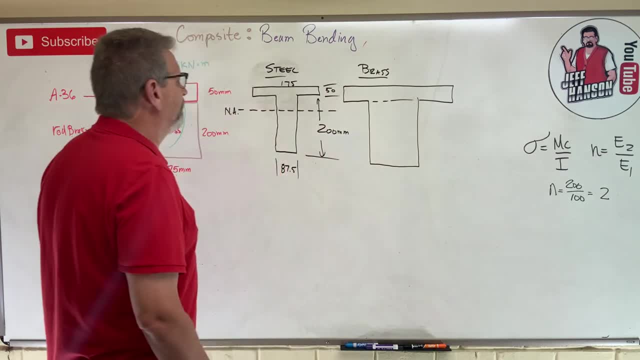 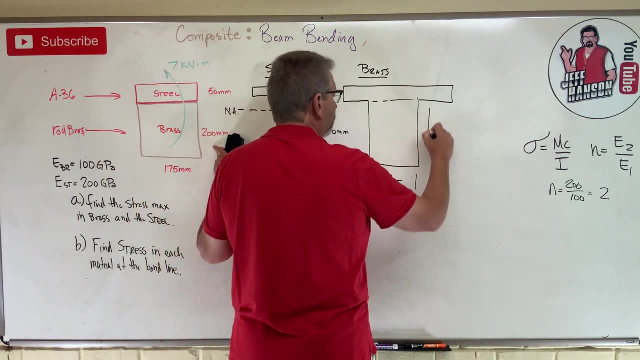 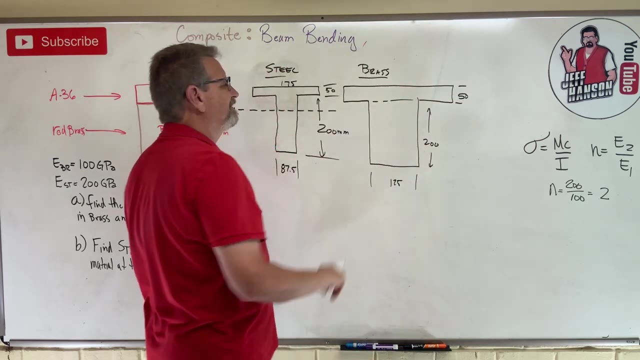 okay. So what is the top up there now? Let's see This over here, 175.. This over here, 200, right, Which means that this over here is still 50, okay, But what's that? So I need twice as much of it, right, Because the brass isn't as strong. So, if it's not as strong, 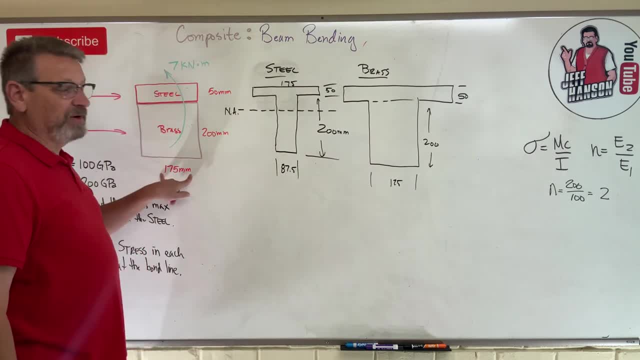 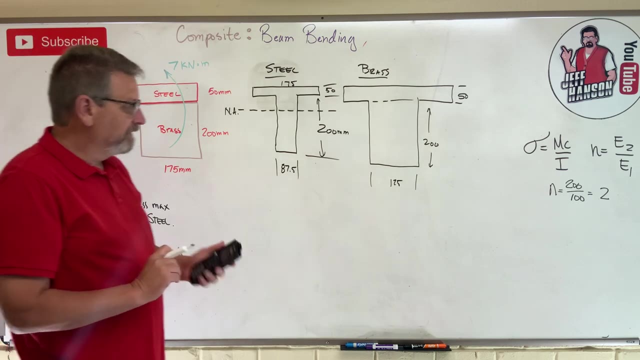 the top width up there. okay, The top width used to be 175,, but I had to make it twice as wide to make it as strong as the steel was right. So what do I get? 175 times 2,? okay, That's 350,. 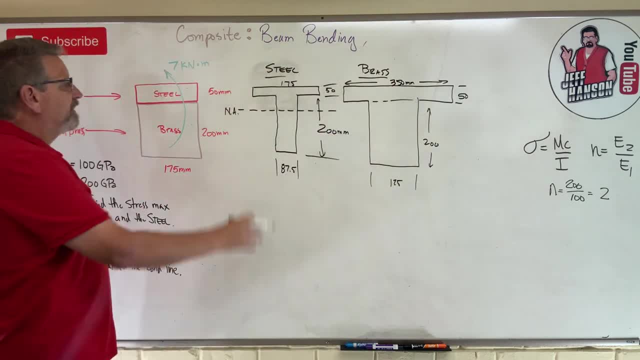 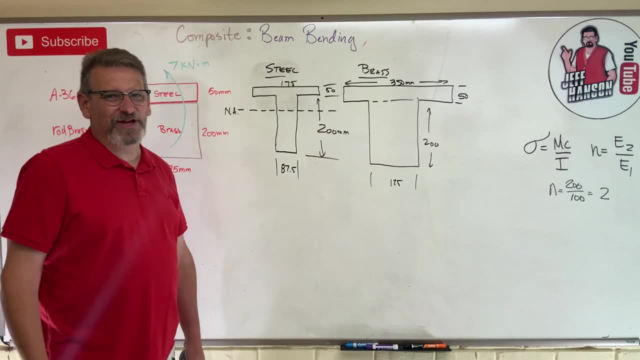 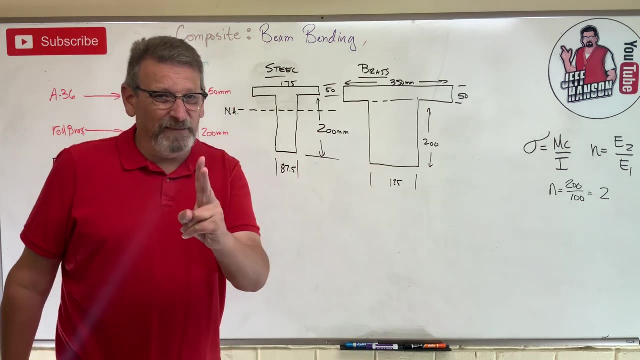 okay, So I can convert it all to steel or I can convert it all to brass, doesn't matter. Get the same answer either way you go. What do you think? Okay, do you know how to do it? Now, here's the only thing that you got to be. here's the only thing you got to pay. 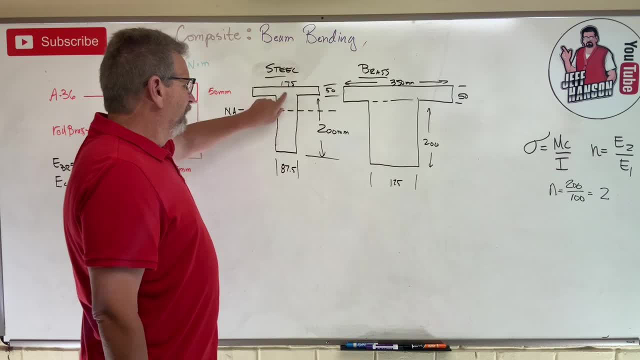 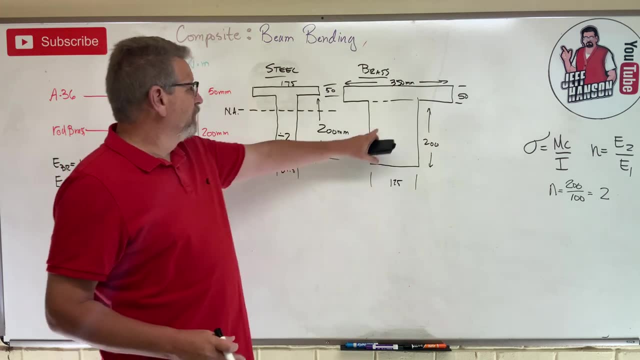 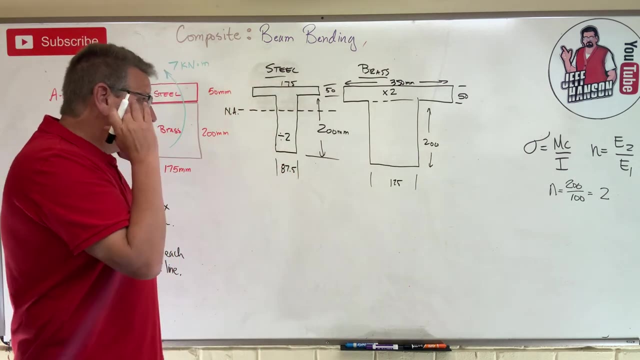 attention to. okay, If you on this one. what do we do? We divided by two, right On this one. what do we do? We multiplied by two, right? Okay, I don't know which one to do, Use your. 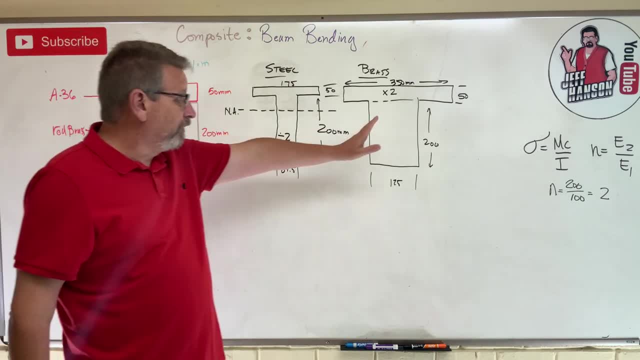 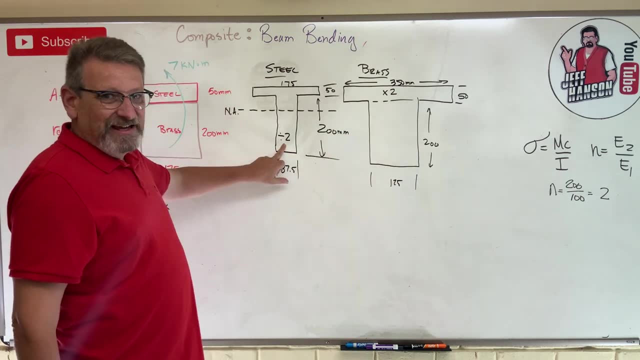 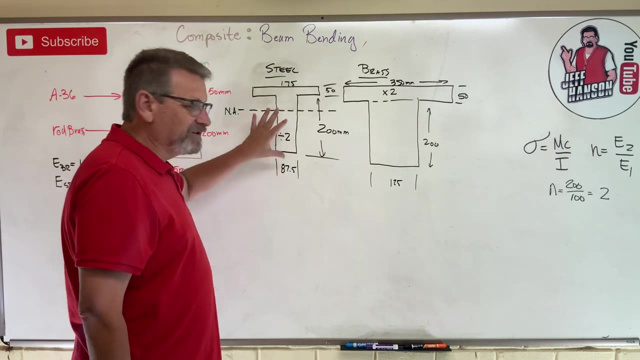 your logic. Just, you can do with logic, The stronger one, I need twice as much of it right To equal the stronger one. So here's the deal. When I get to the very end and I say: what is the stress in the converted material? okay, I calculate it with this new figure. 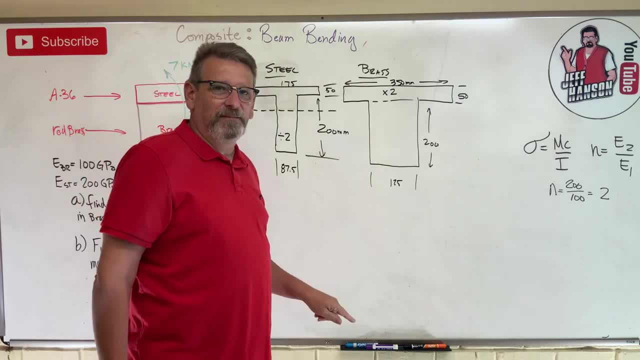 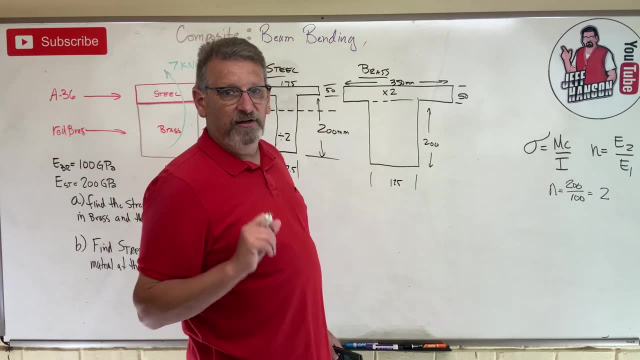 Originally I divided by two, and so when I get to the very end of the problem, I've got to unconvert- okay. So there's the secret: okay, Convert, and at the very end of the problem, unconvert- okay, And you're using this end number right there. okay, All right. so with that, 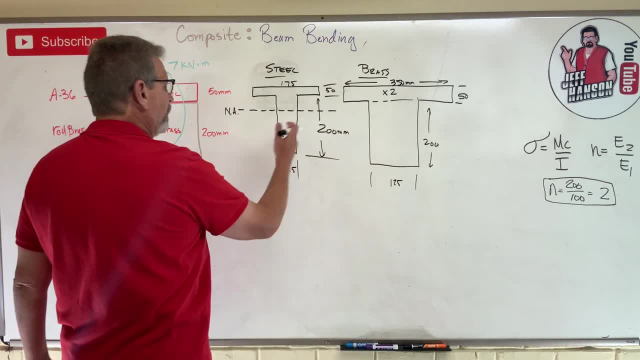 let's see if we can solve this problem. okay, Want to use that one, or you want to use this one? You don't really get to say it: I'm, I'm picking this one. You get the same thing either way you. 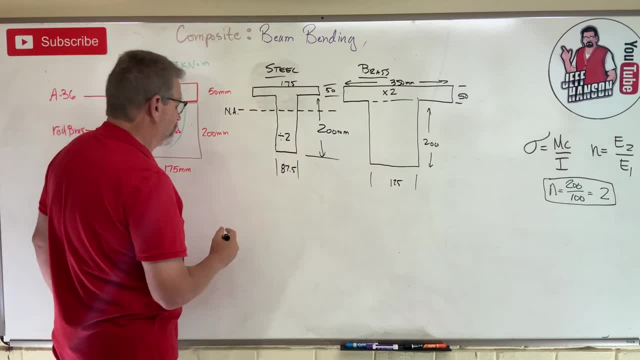 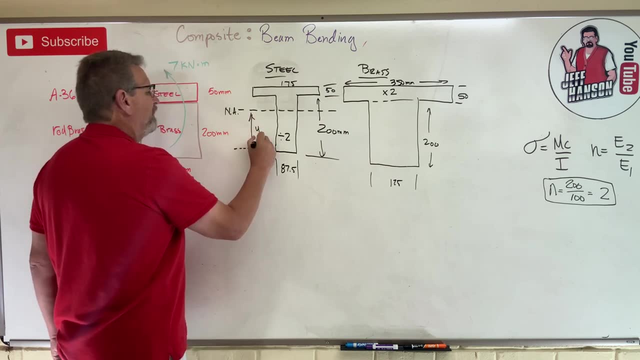 go, but I'm going to pick this one, okay, Just because it's closest to me. okay. The first thing I got to do is I got to find out where in the heck is that neutral axis? You know what It's at some. 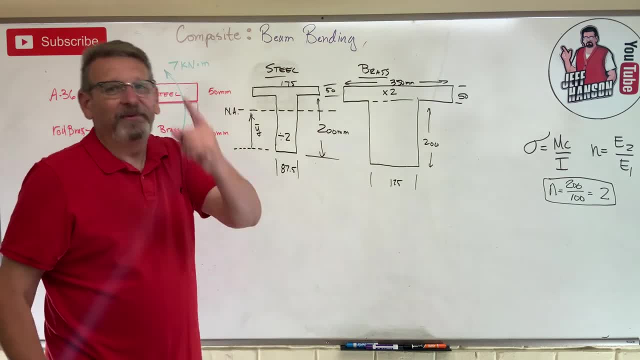 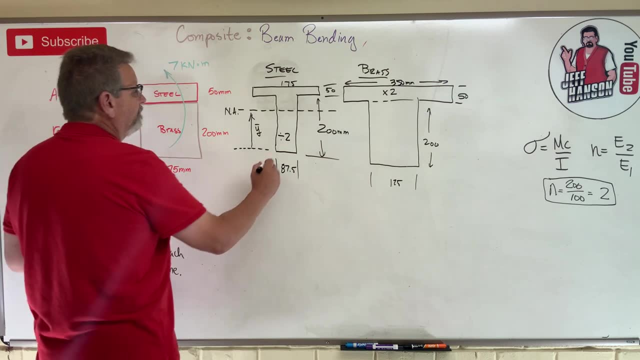 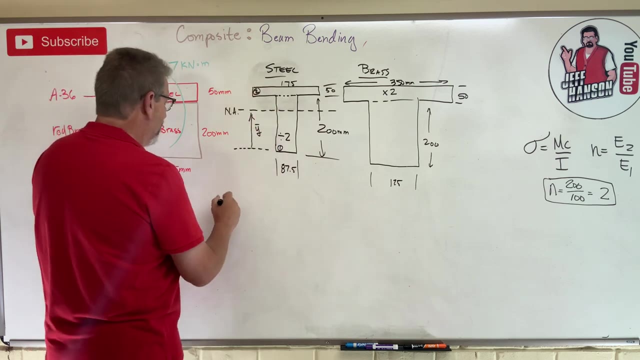 Y-bar. That sounds like a centroid problem. It is okay. You got to go back and do this from centroids, don't you? So here let's make this little thing. here, Let's call this shape one and, uh-uh-uh-uh-uh, we'll call this shape two up here on top. okay, And we got shape one. 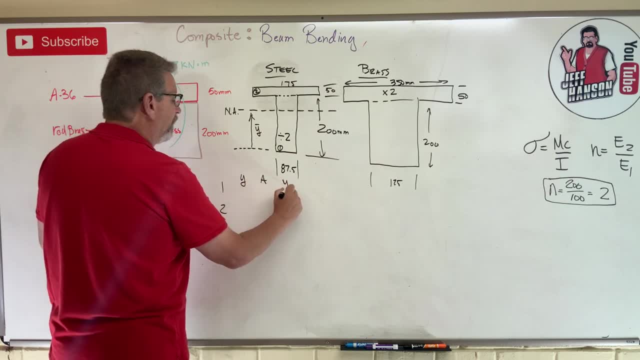 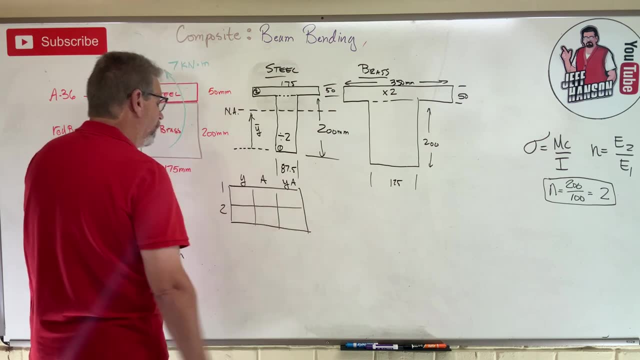 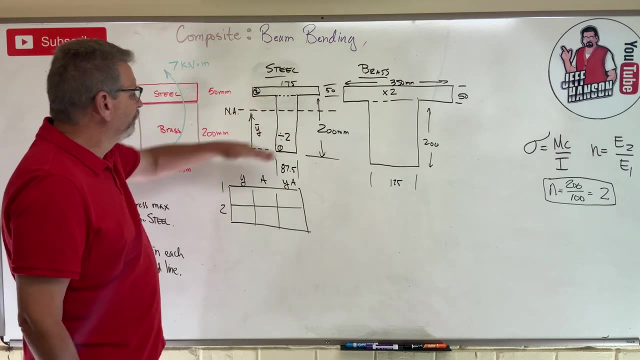 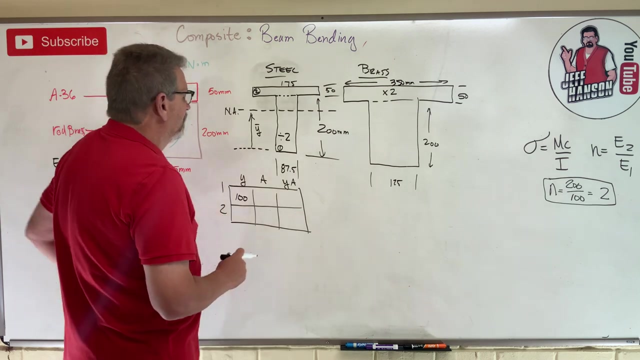 shape two: We got Y, we got A and we got YA. okay, Here we go. Here we go. Shape one: Y-bar. Where is Y-bar for shape one? It's 200 tall, so guess what? 100.. What is A 87.5 times 200, okay, Okay, I should probably be able to do that in my head. 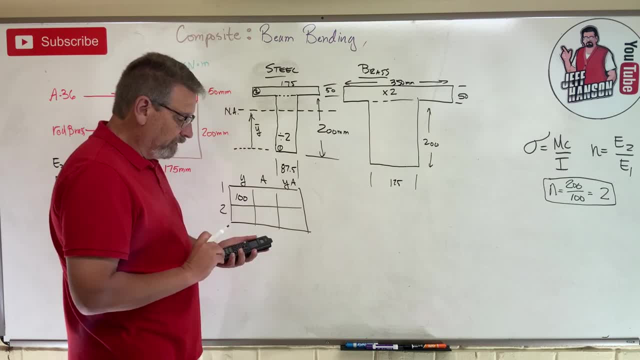 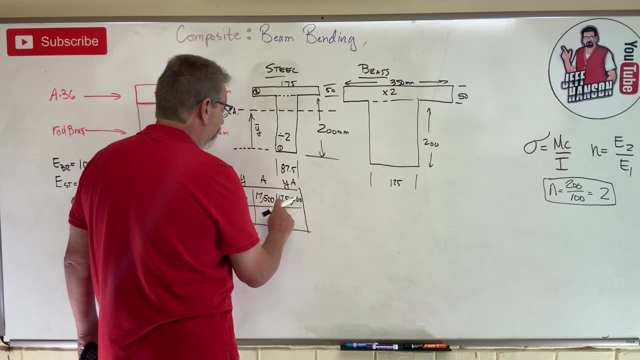 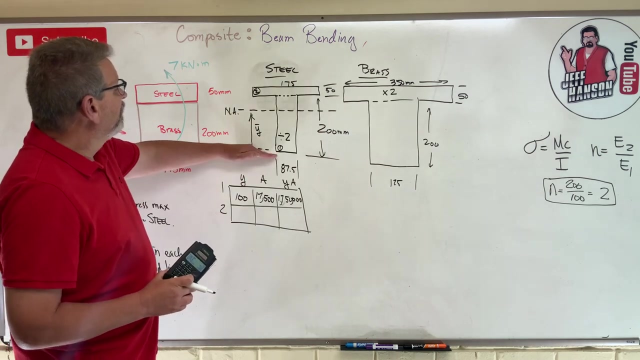 right Times, 200 equals 17,500, okay. And then times another hundred, that's going to be 17, 500, with two more zeros, right, Okay, 1,750,000.. Okay, now shape two. where's Y-bar? You got to. 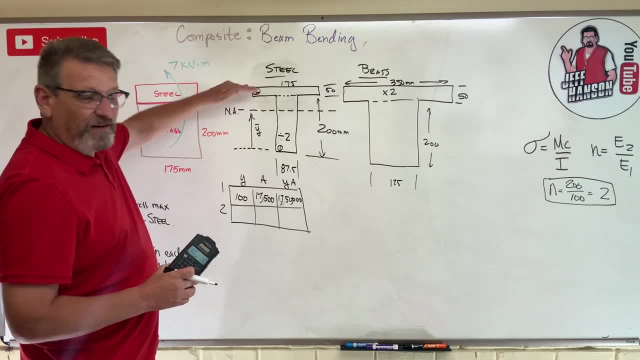 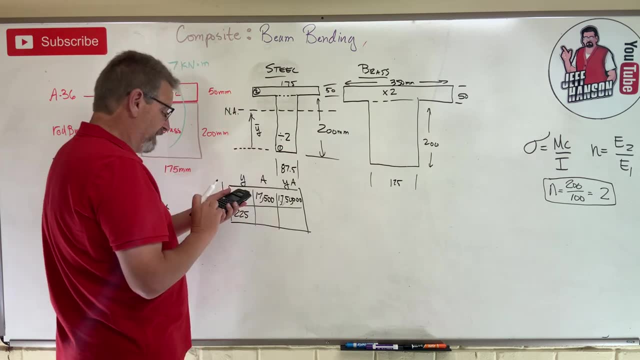 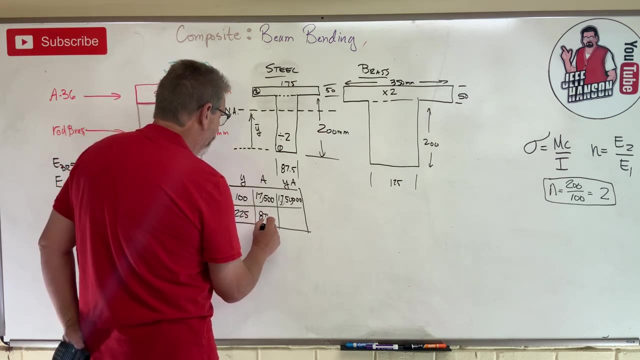 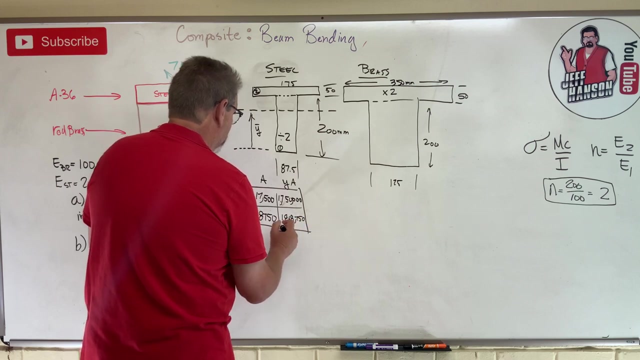 go up 200 to get there, and then 25 more, So 225, and that area is 50 times 175.. 50 times 175 equals 8750.. Okay, Times 225.. Oh, that's big. 1, 968, 750.. Okay, 968, 750.. Yeah, So here we go, Let's add. 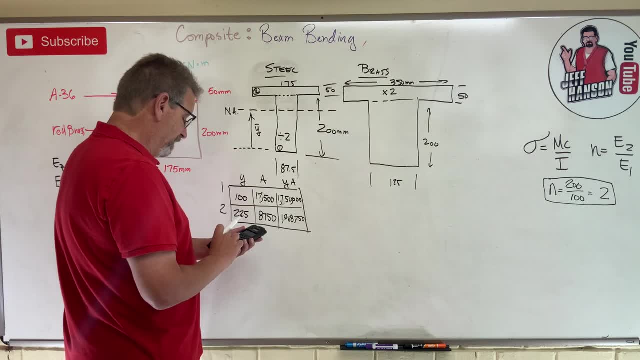 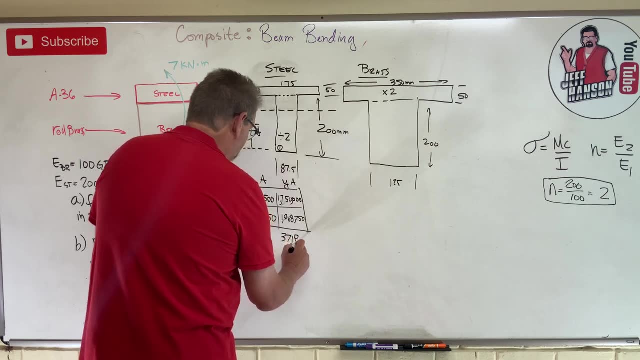 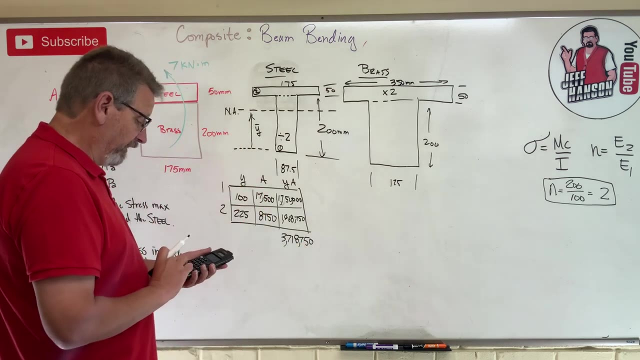 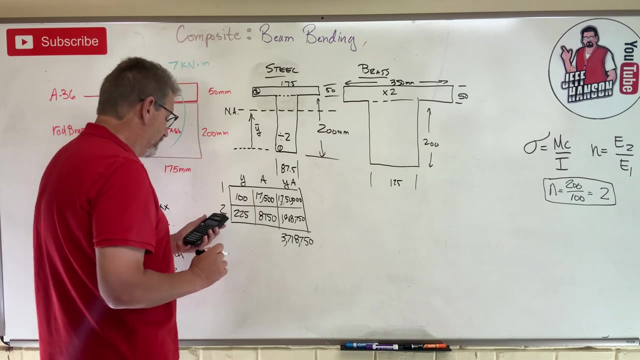 those together Plus 1,750, 1, 2, 3 equals 37,, 1, 8,, 7, 50.. Okay, And these two equal to 17, 500 plus 87, 50,, which is 26, 250.. 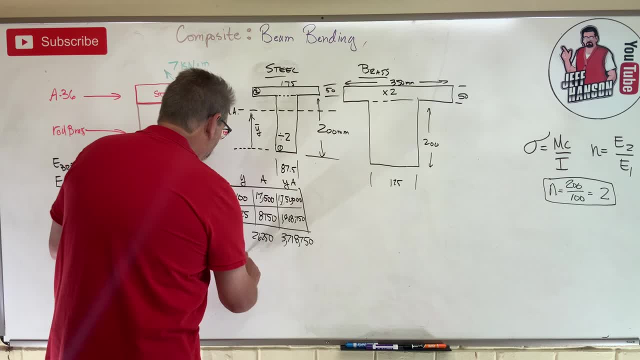 Okay, And so Y-bar is equal to 3, 7,, 1,, 8,, 7, 5, 0 divided by 26, 250.. Okay, And so Y-bar is equal to 3, 7,, 1,, 8,, 7,, 5, 0 divided by 26, 250.. 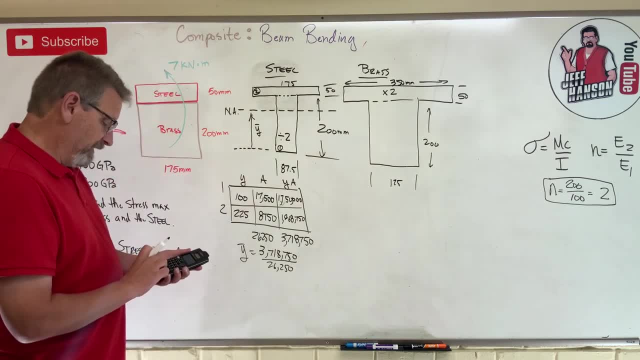 Okay, And so Y-bar is equal to 1, 3, 7, 1, 8, 7, 5,. 0 divided by 1, 2, 3, equal to 37, 1, 8, 7, 5,. 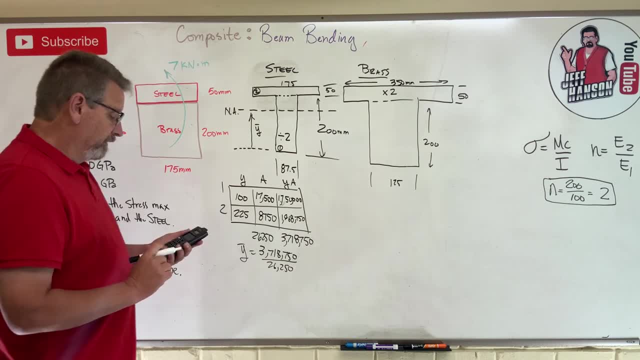 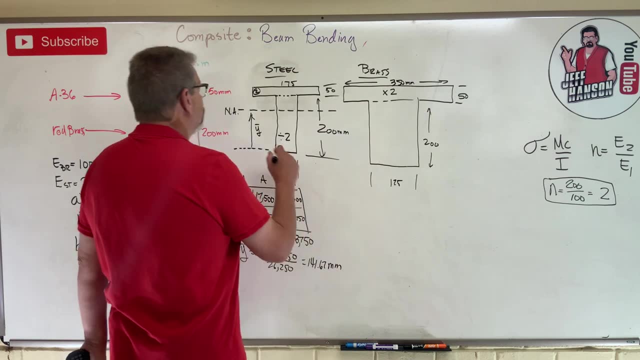 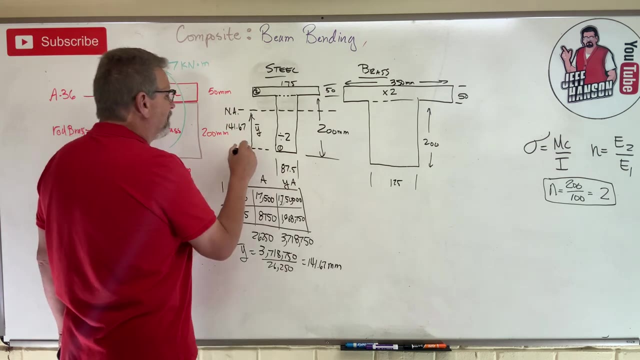 0 divided by 3, 7,, 1,, 8,, 7, 5, 0 divided by answer: 141.67 millimeters. Okay, So from here to here is 141.67.. Now, what I also like to do, then, If I know, from the bottom to the. 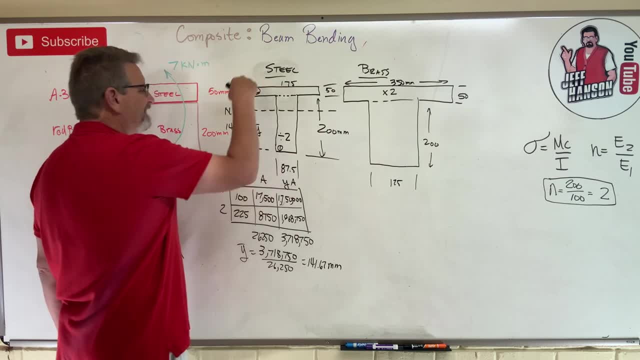 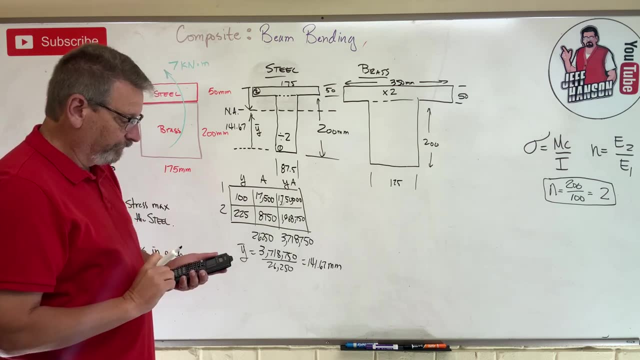 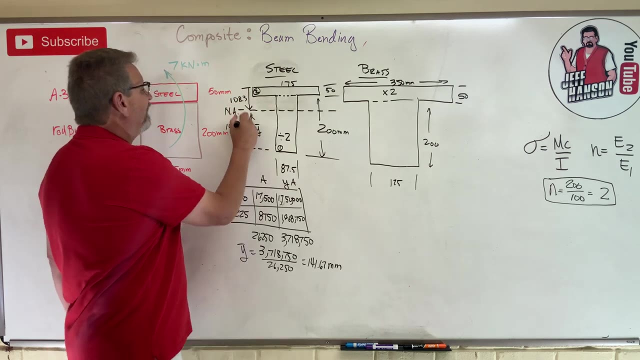 centroid. go ahead and calculate this for me From the top down must be what? Well, it's 250, right? So 250 minus answer equals 108.33.. 108.3, okay, So now I know that distance and I know that. 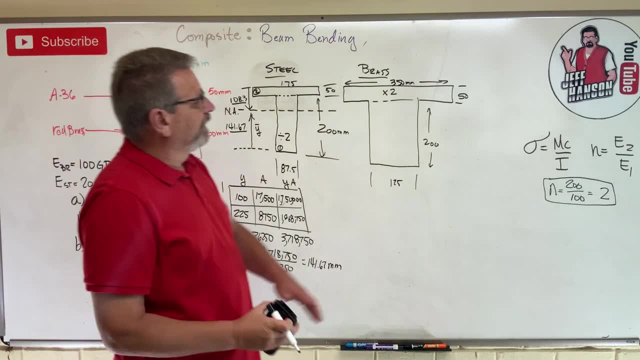 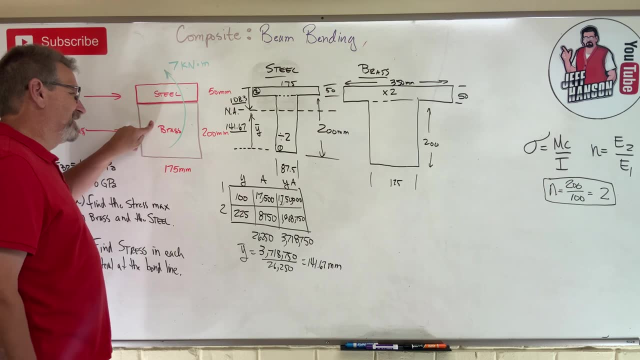 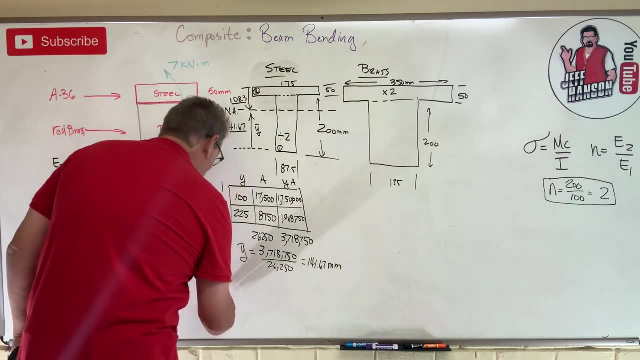 distance, don't I? Okay, Let's calculate I. okay, Now I is going to be for this new shape. It would be nice if it was this shape, because that would be easy. It's just a rectangle, But we changed the shape, So we have to calculate I for this new shape. okay, So I is equal to and remember. 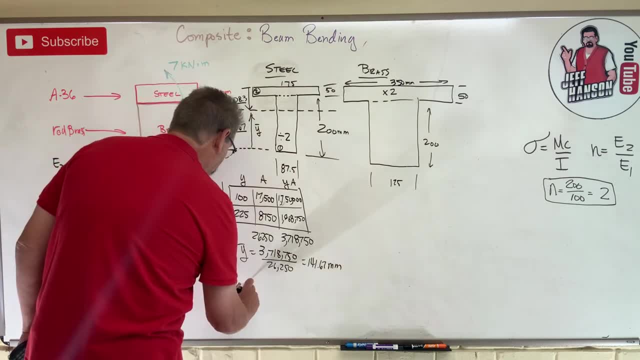 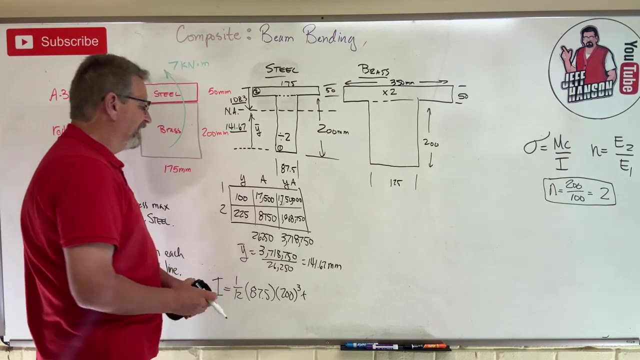 we got two parts, okay, So 1,, 12.. The base of piece number one is 87.5.. And then the height is 200 cubed plus the area of piece number one. handily, I have that already- 17.5.. 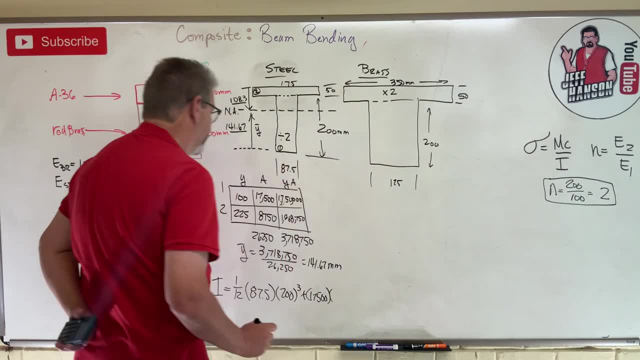 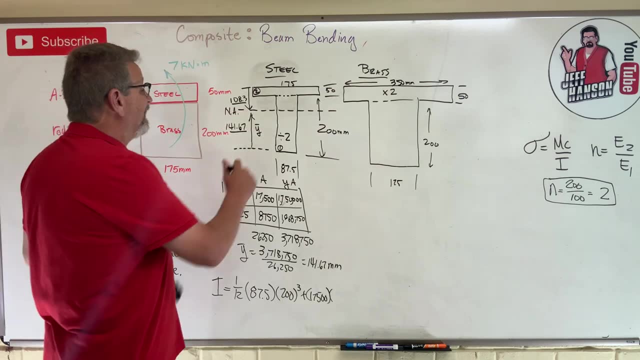 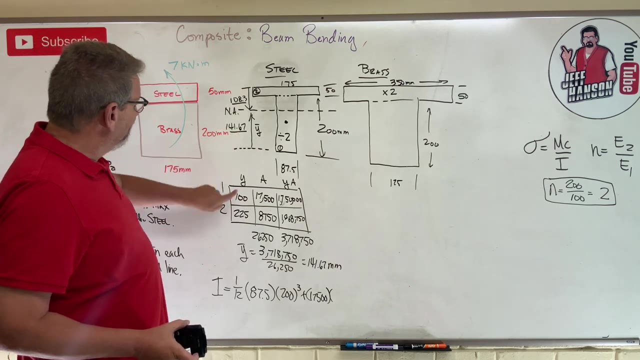 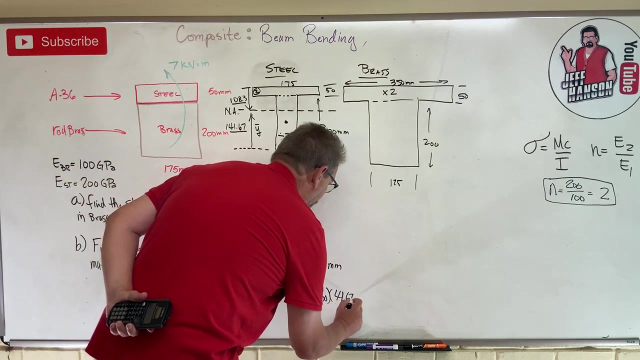 This is the parallel axis theorem. remember, Plus D squared, What is D? Okay, What is D? D is the distance from the centroid of the piece, part to the whole thing there, And it's always this: It's this number minus that number, right? So it's going to be 41.67.. Okay, That's piece number one. 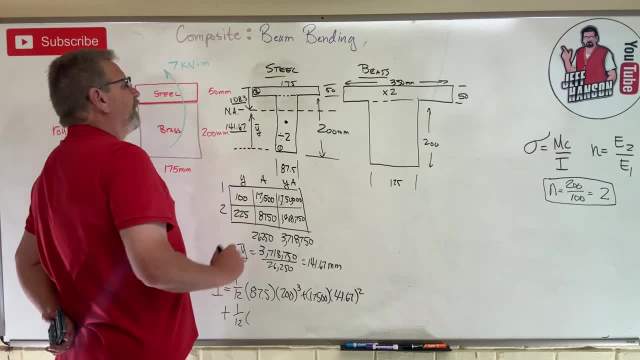 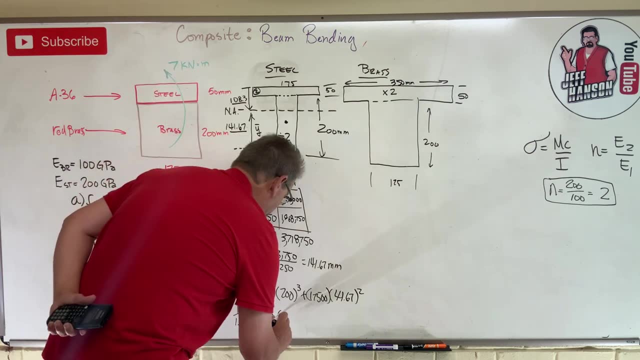 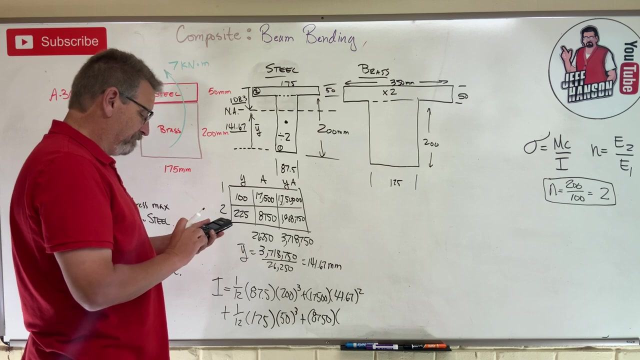 plus, There comes piece number two. It's all about that base. about that base: 175 times the height, 50, plus the area, 87.50.. And then D. What is D? Well, I'll tell you what it is: It's 141.67 minus 225 equals 83.33.. 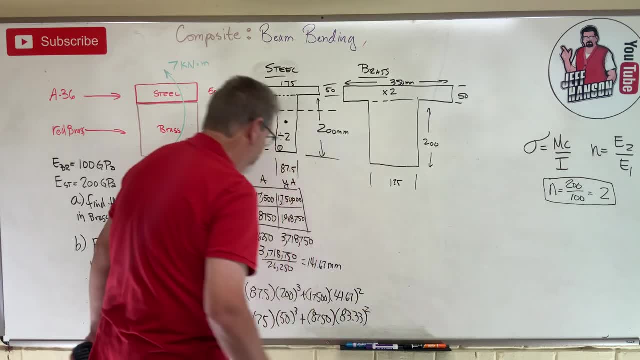 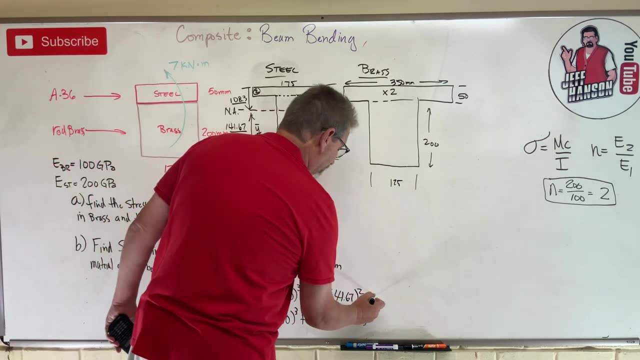 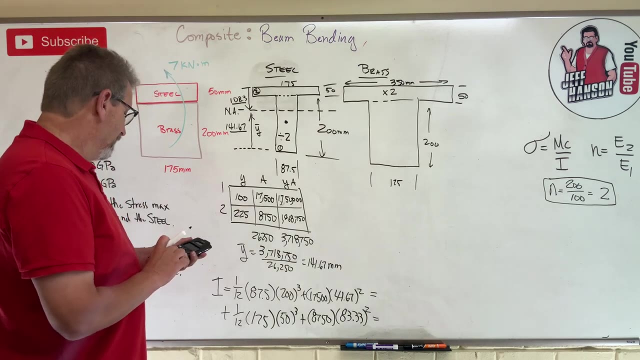 Okay, Let's add those together. Now, this is in millimeters, So it's going to be a big number. Are you scared? I'm not scared. Okay, Let's see what we get: 87.5 times 200 cubed equals. 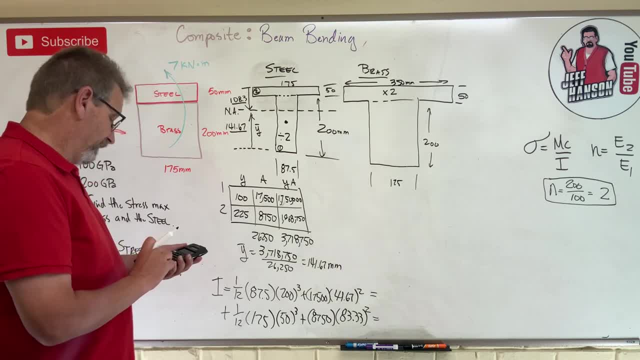 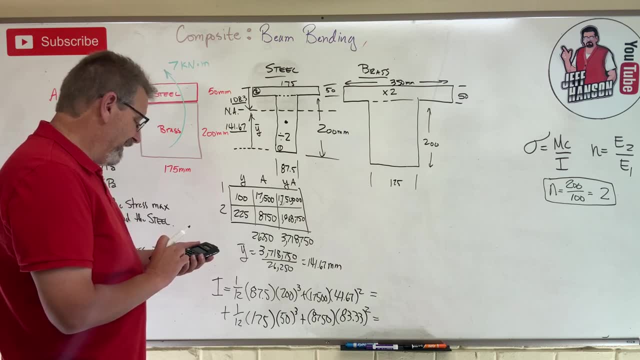 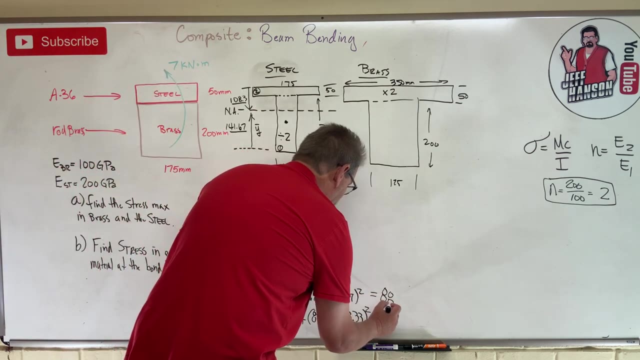 divided by 12 equals plus 17,500 times 41.67.. 267 squared equals: woo, that's a big number. I'm gonna add this one to the next one: 88, 720,, 139, .08, okay, now that's millimeters. 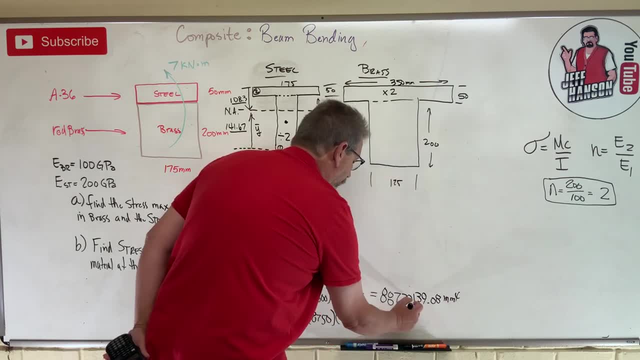 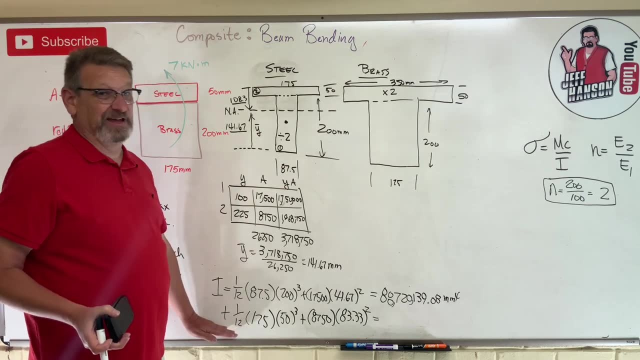 to the fourth, but that's only for piece number one. okay, I like to calculate these separate because I find that students put these in their calculator kinda poorly and mess up on the calculation on. you know, don't lose points on calculator error, right. 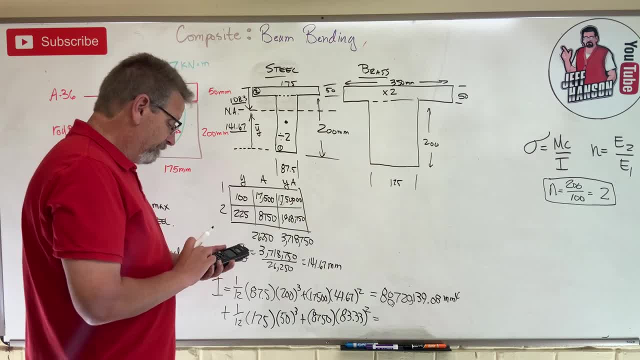 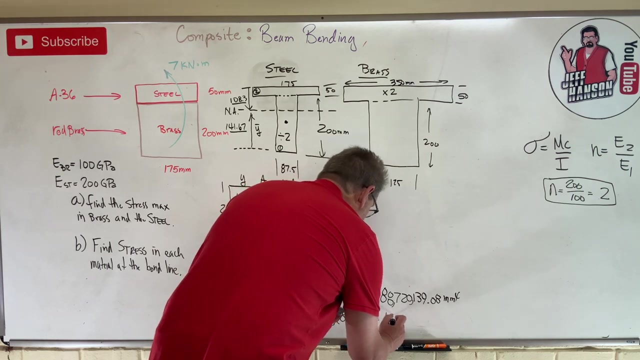 175 times 50 cubed equals divided by 12, 12, equals plus 8750 times 83.33 squared equals- 83.33 squared equals. Okay, here's another next number: 62581944.5, so let's add that to that other one. 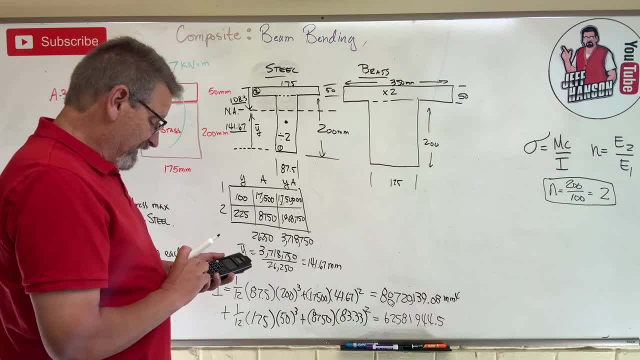 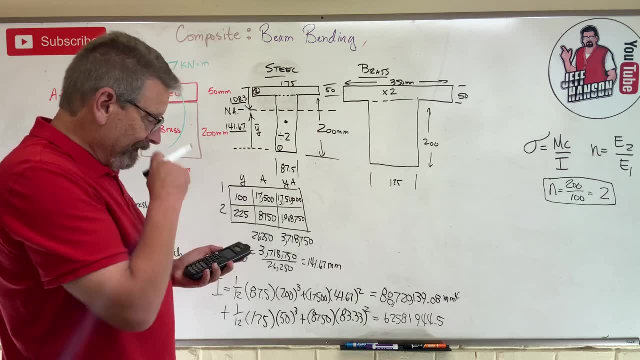 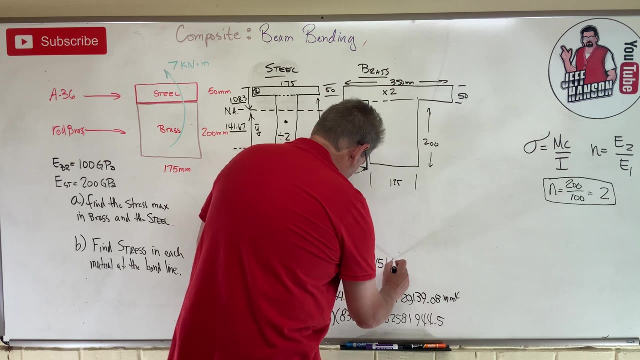 So plus 88, 720,, 139.08 equals. Okay, here's our I. I equals 151302083, don't forget .6,. okay, there you go. So 151 million millimeters to the fourth, okay. 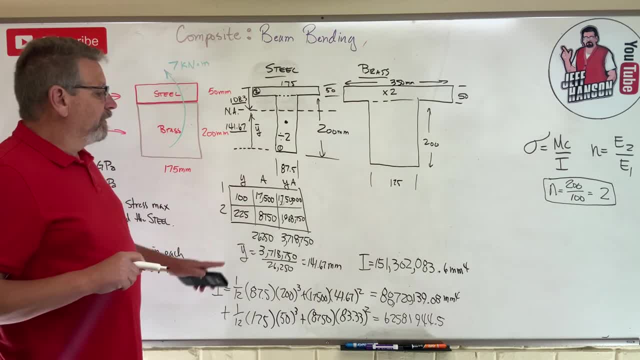 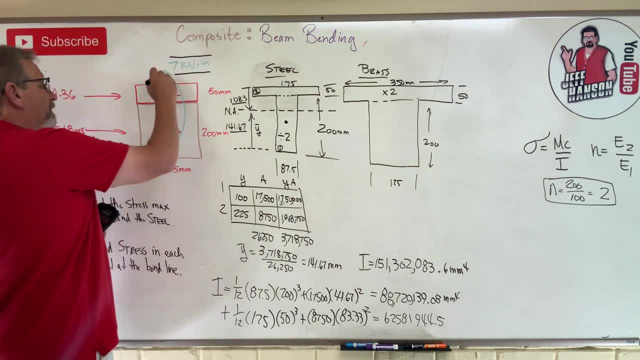 Woo, that's big. All right, we got that. Do we know? M? M is given on this problem, okay, And they just gave us this our big, big bending moment. okay, This is the moment across that beam like that, right. 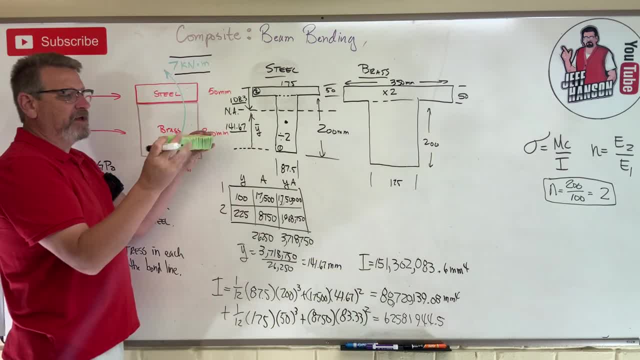 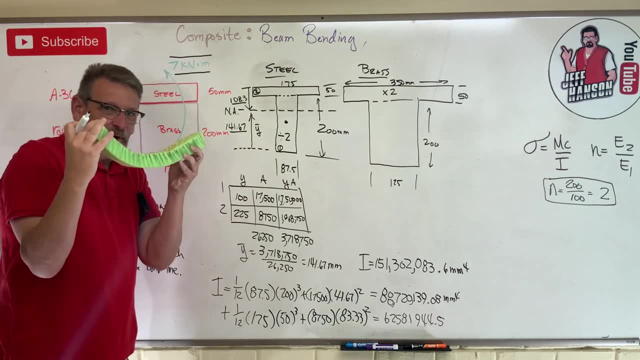 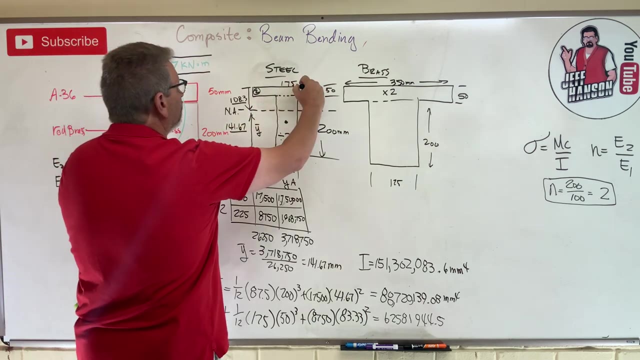 So we can think about that beam coming out at you, right? That bending moment is like this: So it's putting the top in compression, isn't it okay? The top is in compression, okay. So everything up here is gonna be compression. 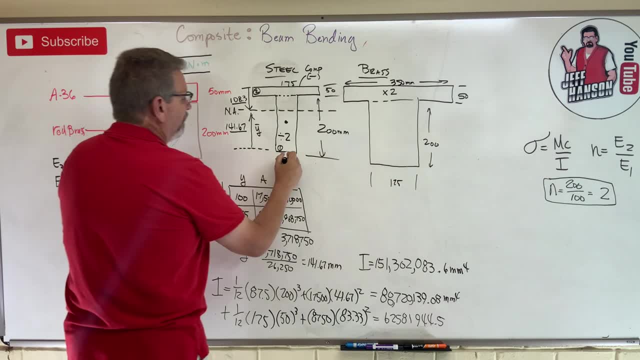 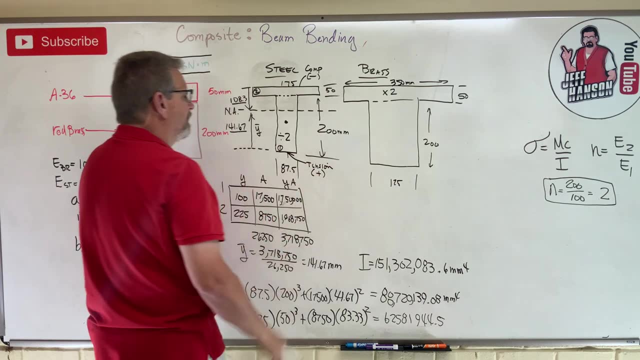 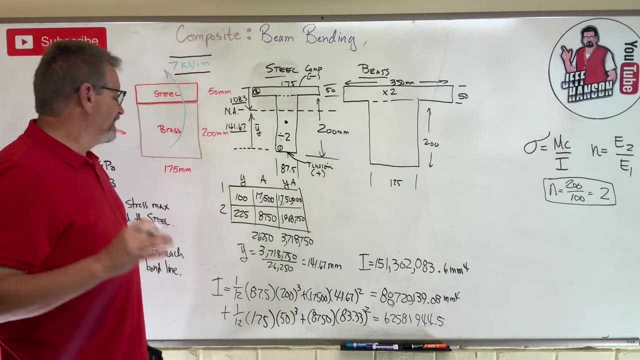 which the stress is gonna be negative, right. So everything on the bottom down here is gonna be in tension, Right, And so the stress down here is gonna be positive, okay, All right. So I think now we're ready to calculate some stress. 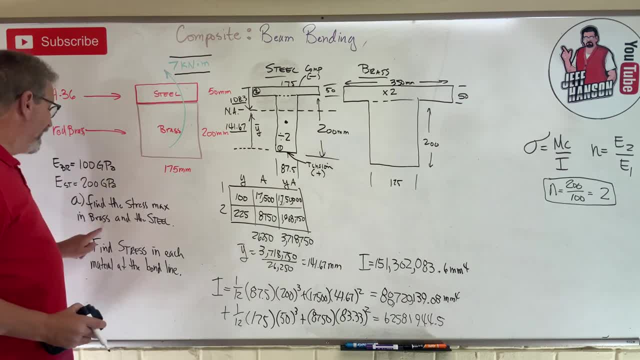 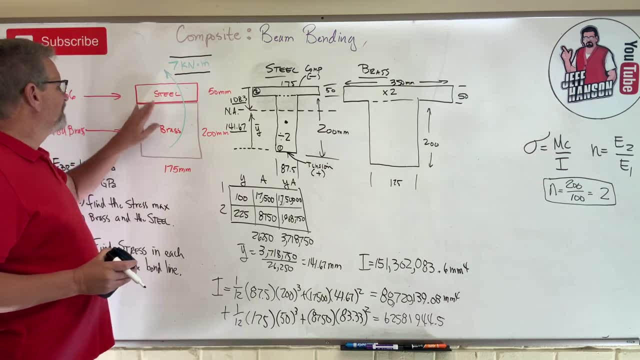 because what we're gonna do? find the stress max in the brass and the steel. okay, The worst case, brass. okay. now the brass is on the bottom and the steel is on the top. So the worst case for the steel, where's it gonna be? 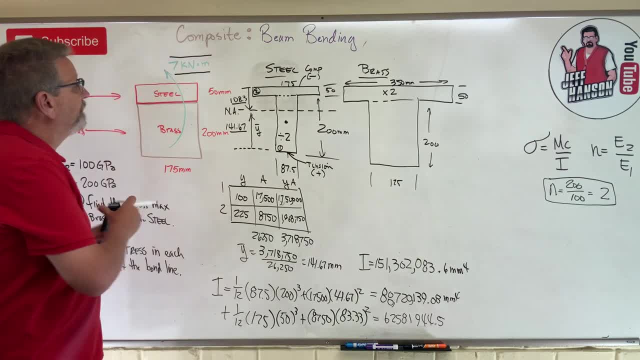 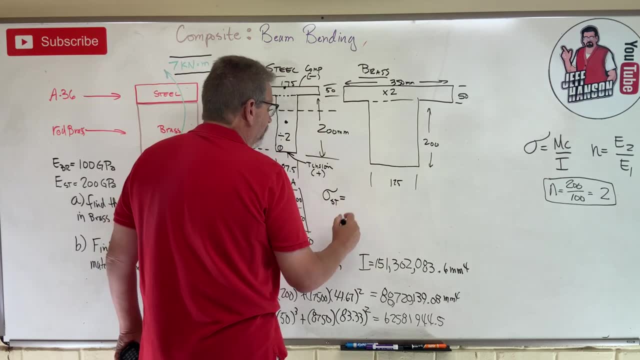 As far away as I can get right. So the steel is gonna be up here on the bottom right, It's gonna be up here on the very top. okay, So here we go. Sigma steel is equal to bending moment of 7,000,. 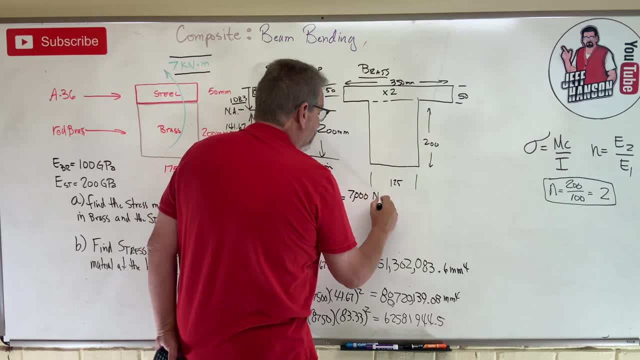 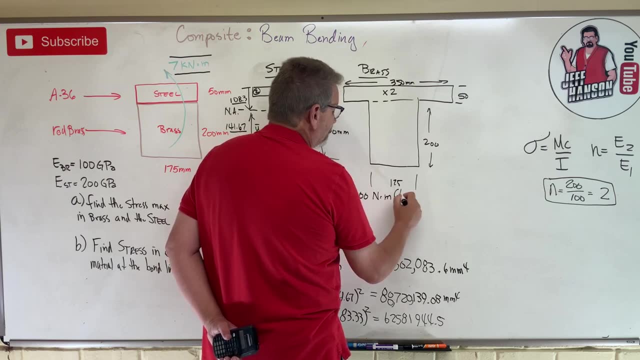 I just got rid of the kilo right there. right, Newton meters. now this down here was in millimeters, so I'm just gonna convert it, okay. So a meter is 1,000 millimeters, okay, Times C. 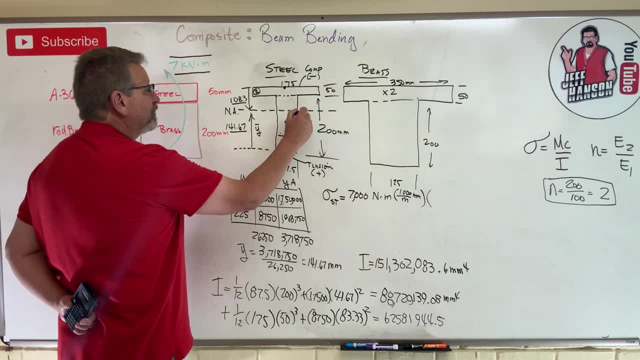 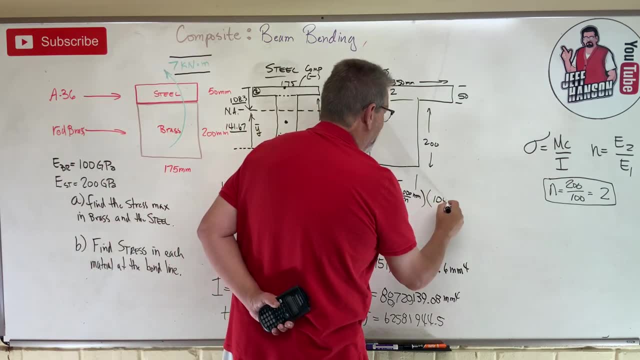 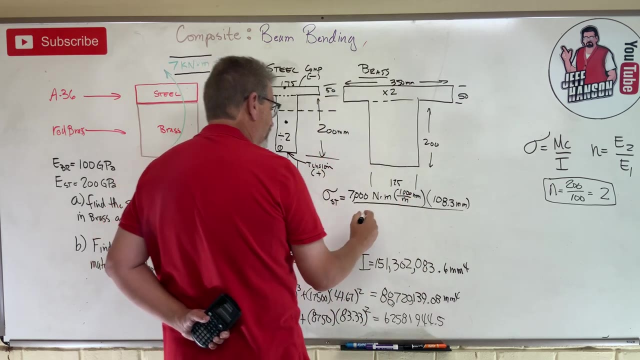 What is C for the steel? That would be from the neutral axis to the outside of the part, which is 108.3.. 108.3 mms all divided by I, which is this ginormous number down here: 151, 302, 083.6 mms to the fourth. okay, 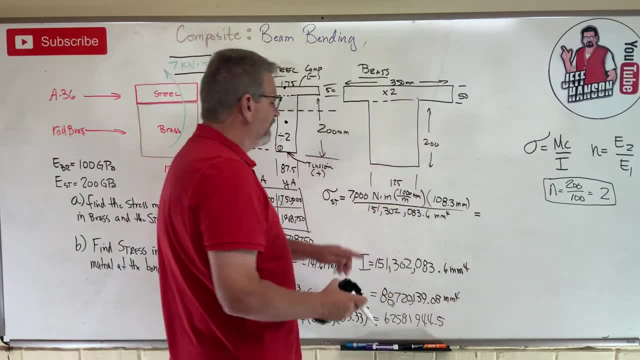 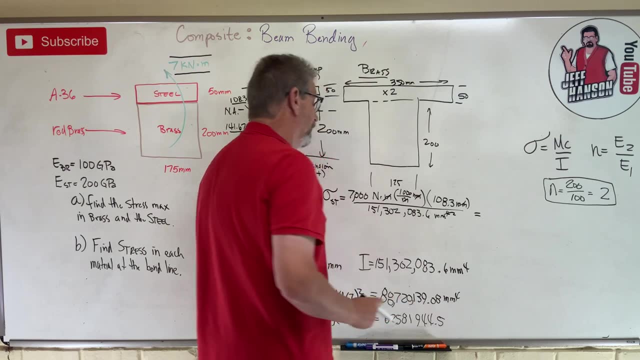 So let's see what that is: Equals. now what are we gonna get here? We got newtons right, Meters canceled out. We got a millimeter and a millimeter. that leaves us with square millimeters: Newtons over millimeters squared. 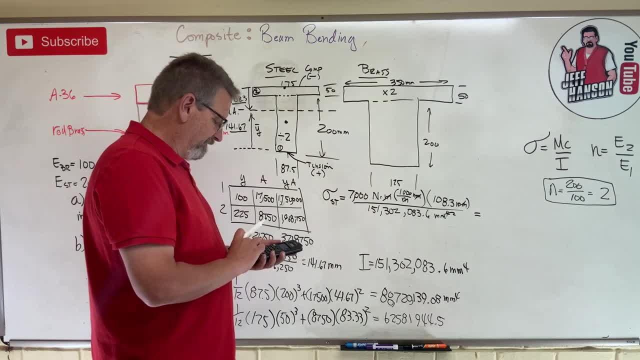 That's a megapascal, isn't it? So here we go clear. 7,000 times 1,000, whoop Times 108.3.. Equals big: divided by 151, 302, 083.6, equals 5.01.. 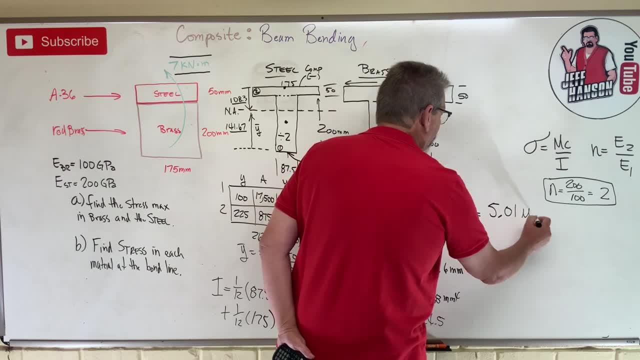 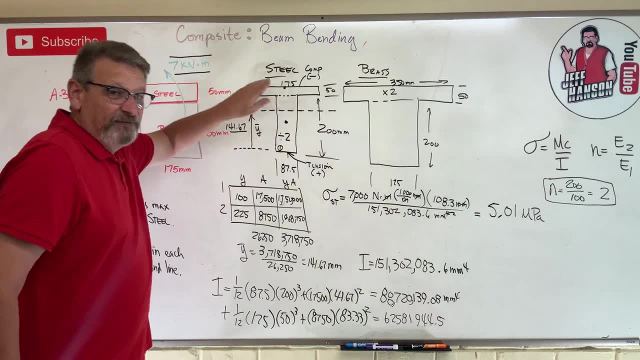 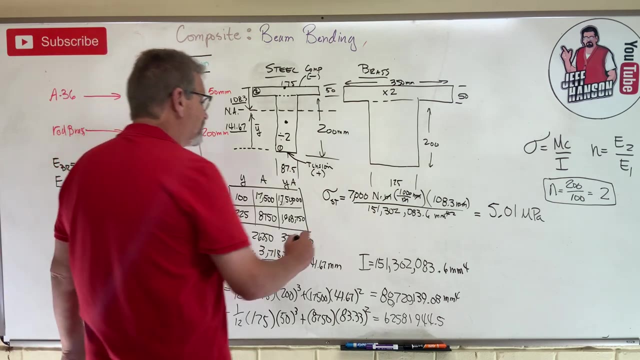 All that, that equals 5.01,. okay. Now do I have to unconvert that? No, because I never converted the steel, did I? I converted the brass. So now let's find the brass. okay. So sigma for the brass, what's it equal to? okay? 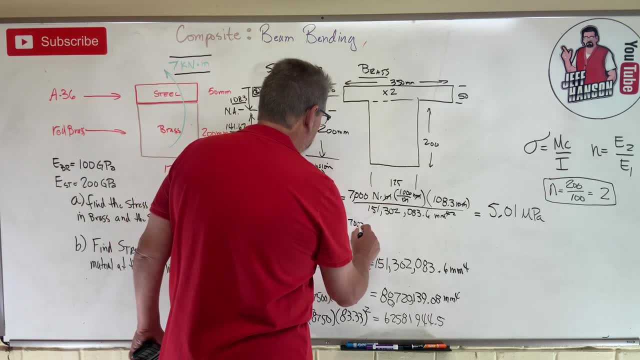 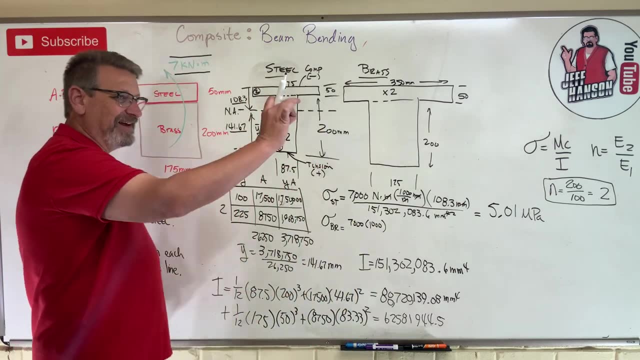 Guess what? Same bending moment: 7,000 times 1,000.. That'll unconvert it to millimeters, right. And what is C? the distance from the neutral axis to the worst brass particles. Well, the worst brass lives down here. 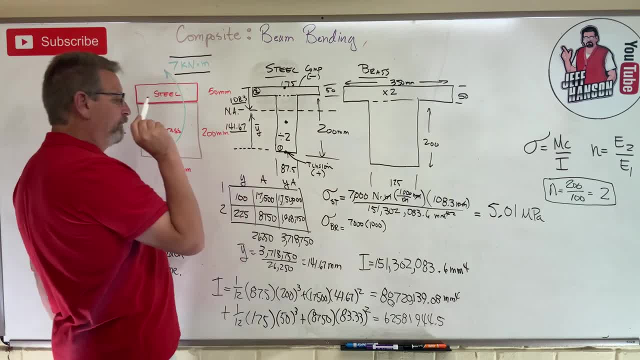 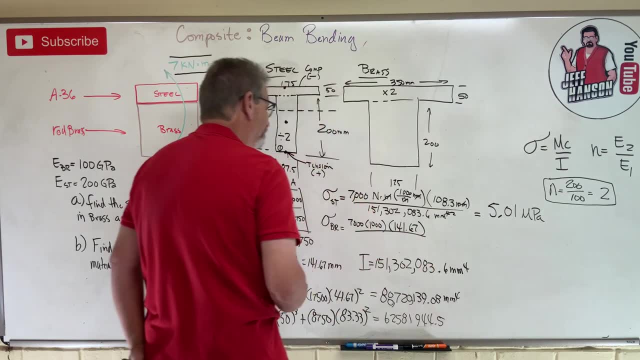 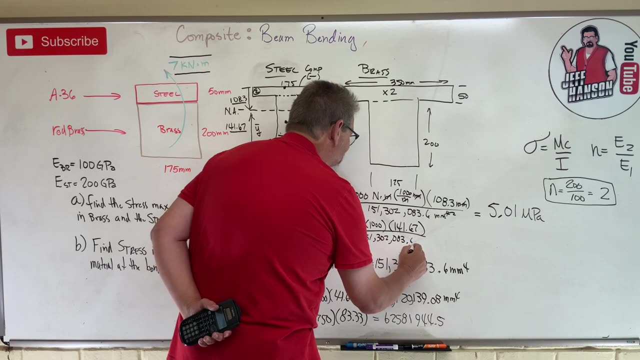 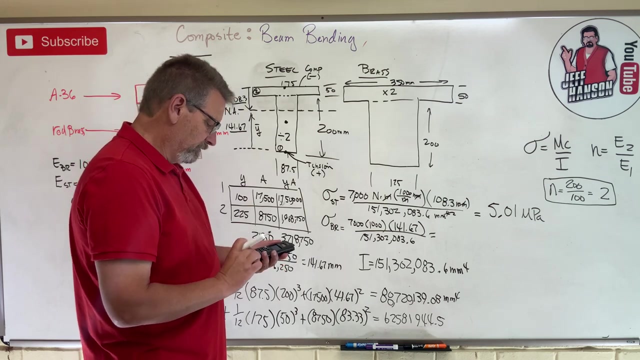 on the very bottom of the part. So I'm gonna go 141.67 to get down there. So times 141.67 divided by 151, 302, 083.6,. okay, Equals here we go: 7,000 times 1,000, times 141.67,. 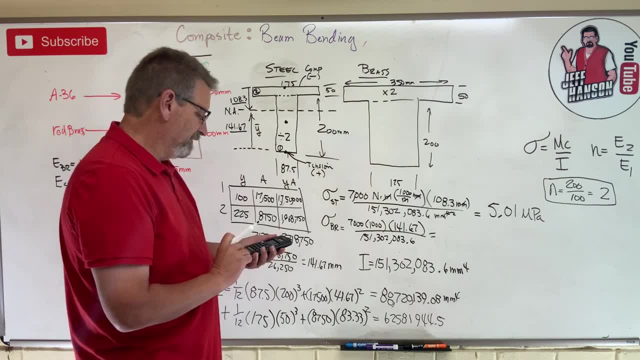 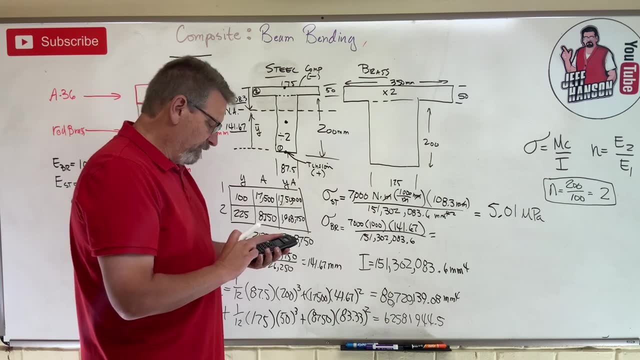 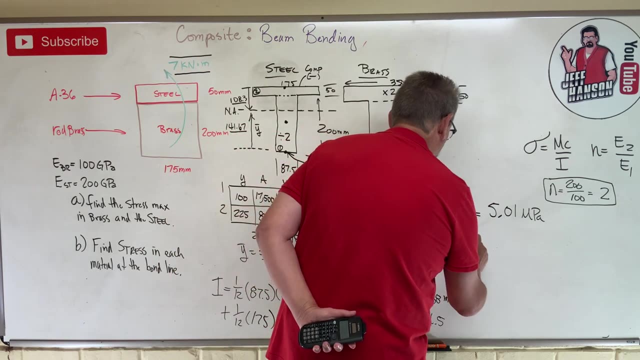 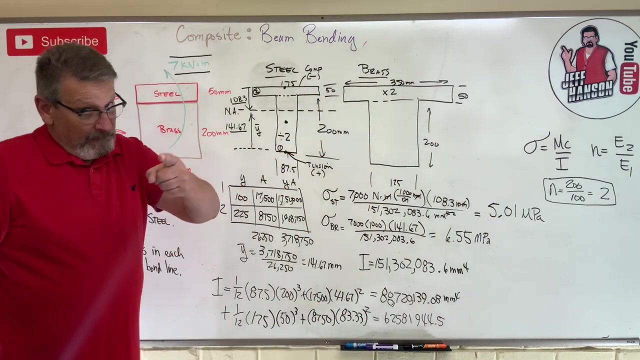 equals divided by 1,000, times 1,000, 302, 083.6,. okay, Equals 6.55.. Now is that the stress in the brass? The answer is no. okay, I divided by two. 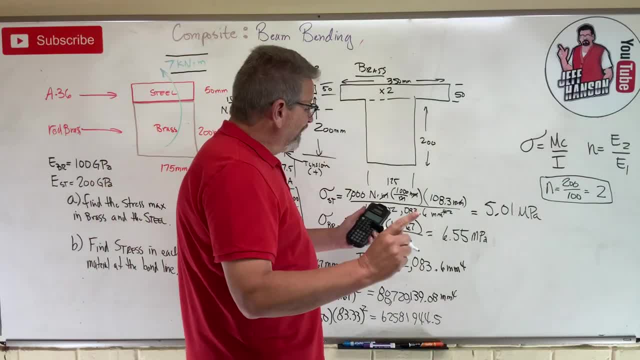 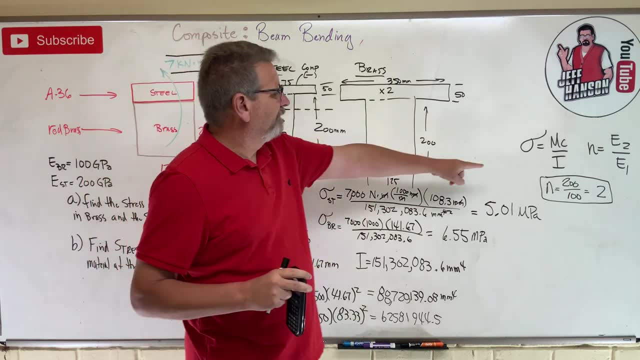 So what do I need to do to that guy? All right, so here's the important thing is now 6.55,. I was calculating the brass. Here we go, here we go that as if it was steel, but it's really brass. And brass is what? Brass is half as much as steel. 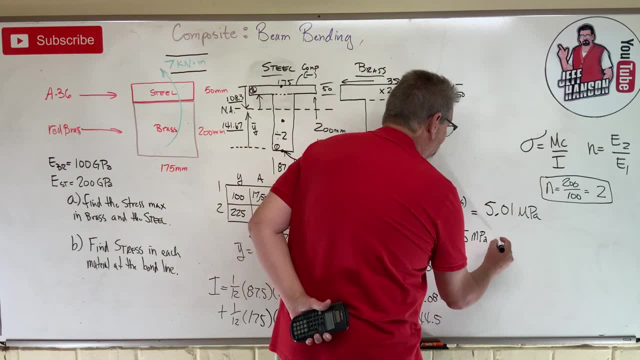 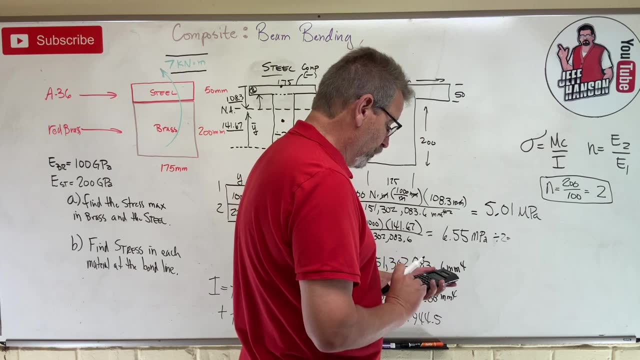 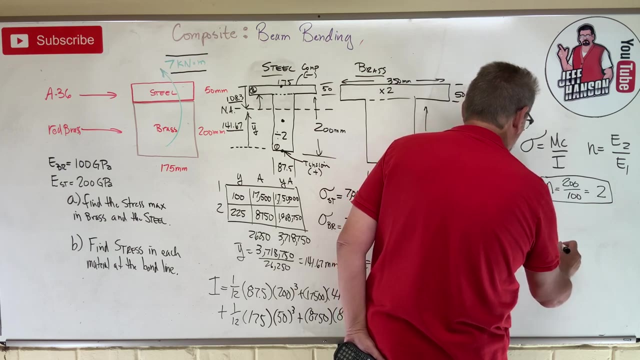 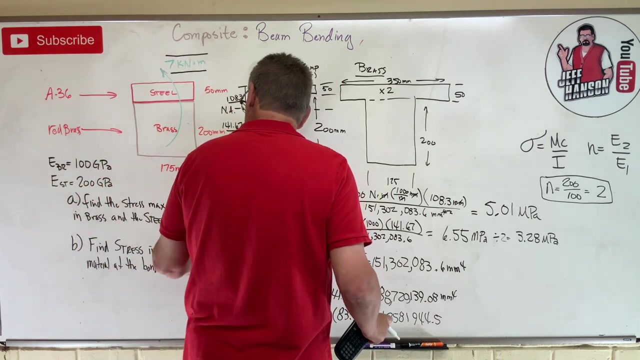 isn't it? So I need to take this guy here and I need to divide by two. So the brass is what? 6.55 divided by two, 3.28.. Okay, One more step, and that is this Part B. find the stress in each of the materials at the: 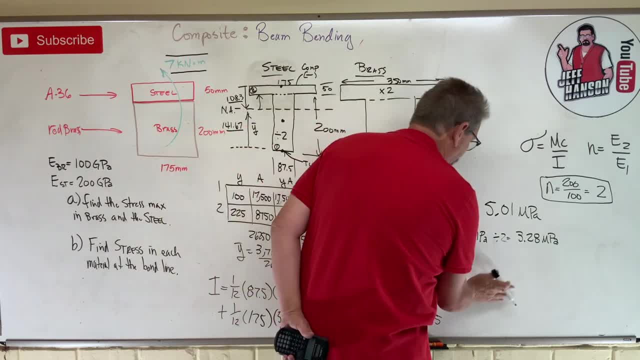 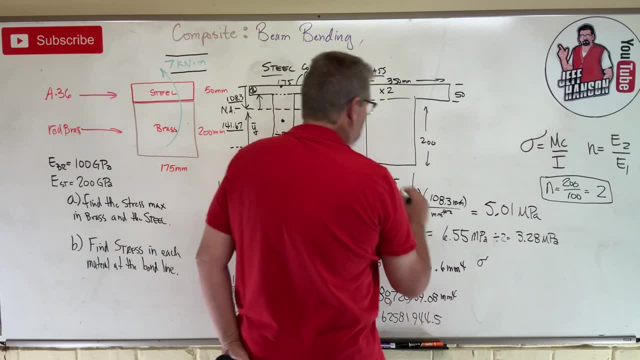 bond line, So not at the top of the part or the bottom of the part, but at the bond line. Okay. So what's that going to be? Let's do sigma steel, right Steel at the bond line. Okay, So that. 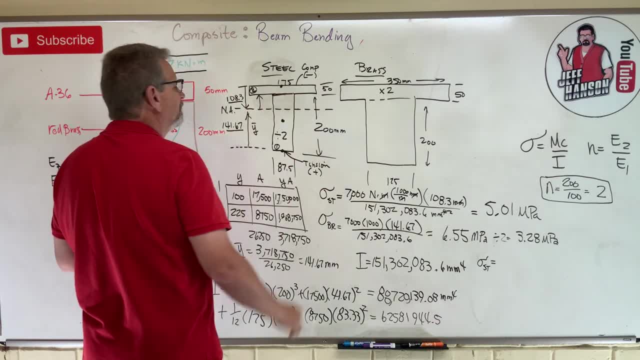 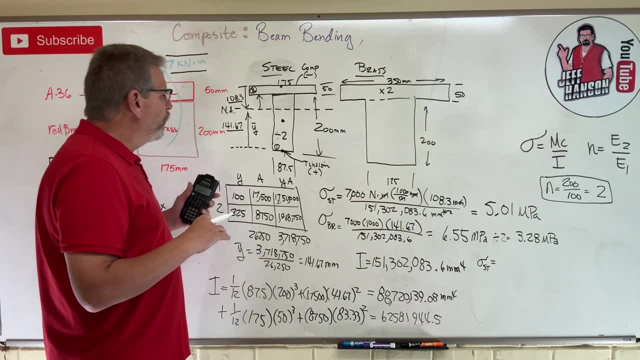 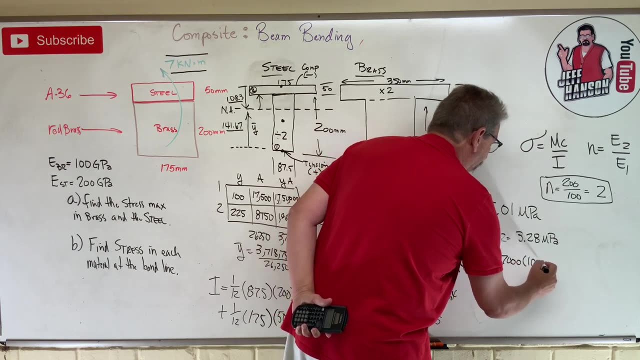 here's the bond line, right here, where they're glued together. however, they're connected right. Maybe they're explosively welded or something cool, I don't know. Okay, So guess what? The bending moment: same thing 7,000 times, 1,000 times C. What is C at the bond line? Well, 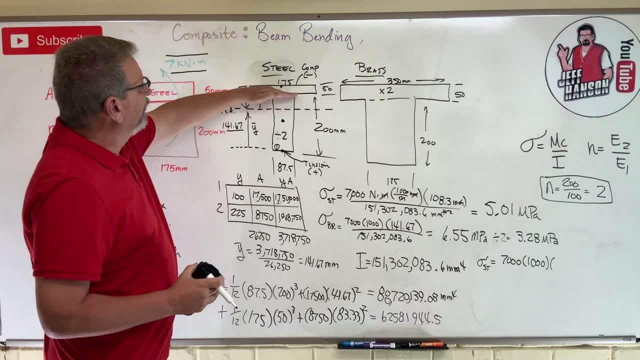 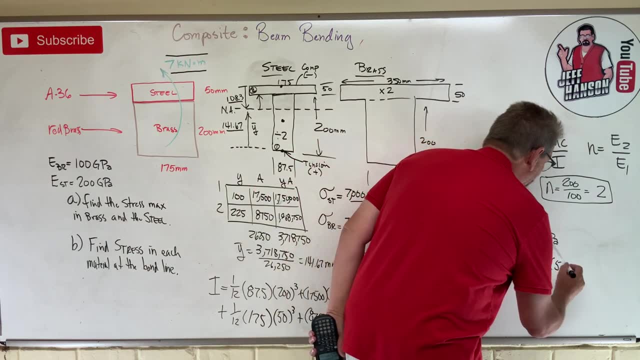 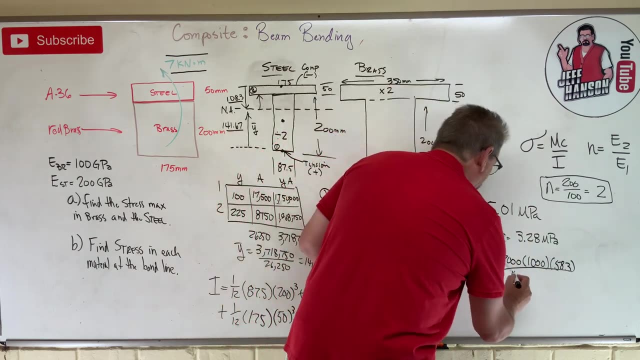 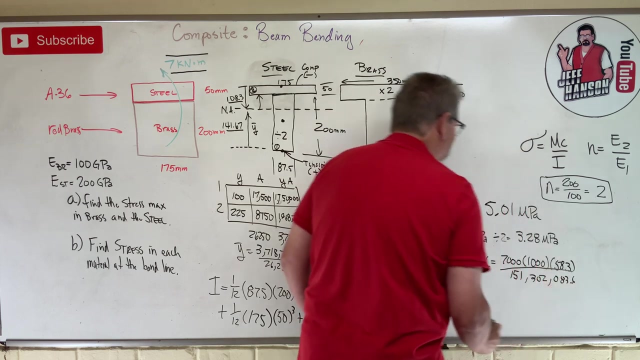 from here to the top of the part, it's 108.3.. So, from here to the bond line must be that minus 50, 58.3.. Okay, Divided by same moment of inertia, giant number 1, 5, 1, 3, 0, 2, 0, 8, 3.6..